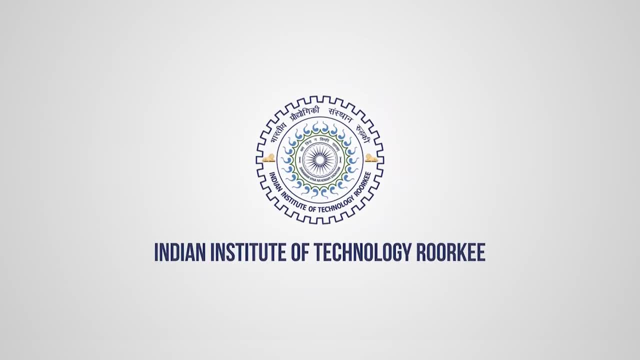 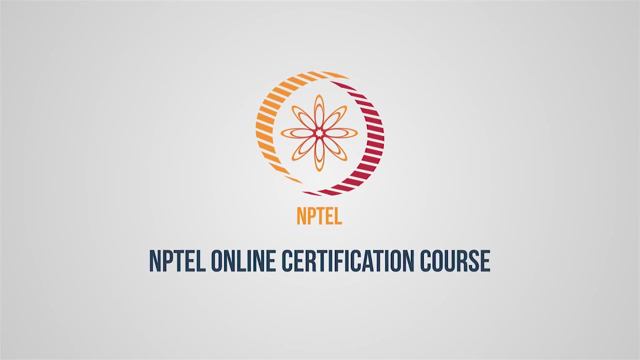 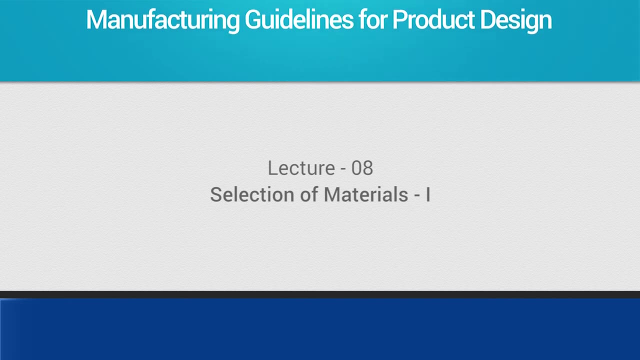 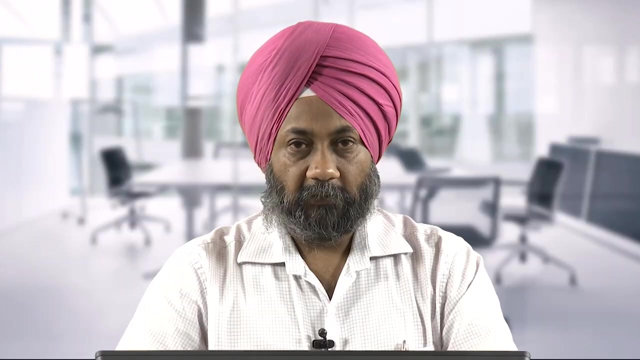 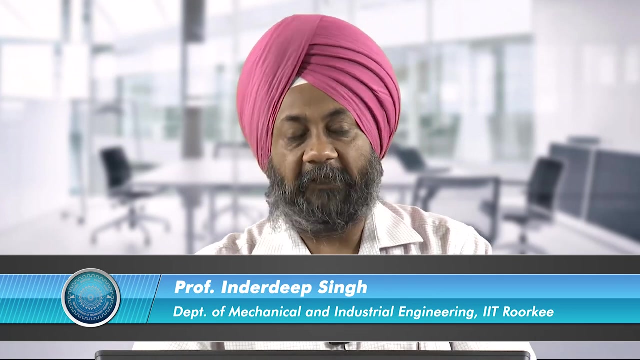 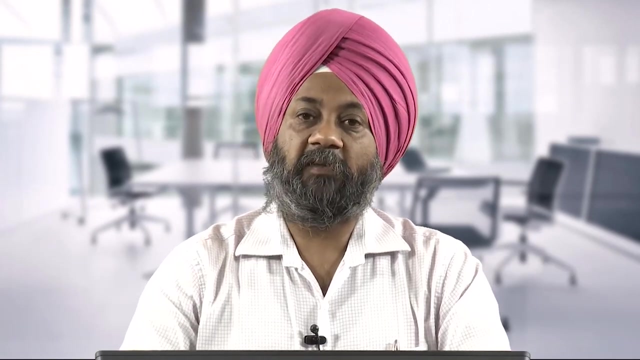 Namaskar friends, welcome to session 8 of our course on manufacturing guidelines for product design. We are currently in the second week of our discussion and, as you are well aware, our focus in the week second is on engineering materials, because all of us know that, for any product, 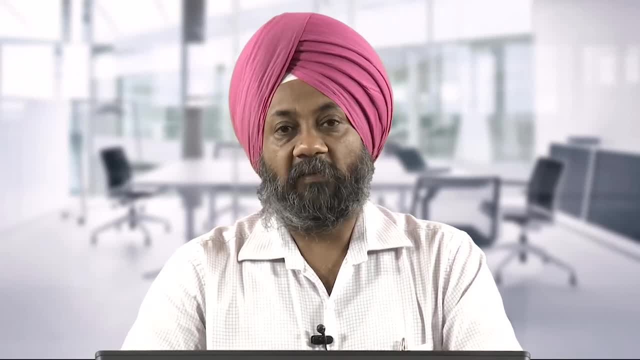 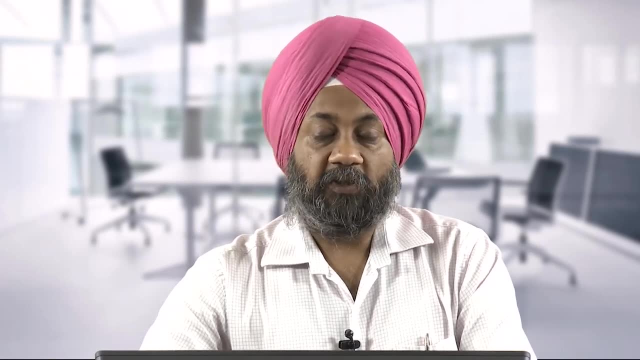 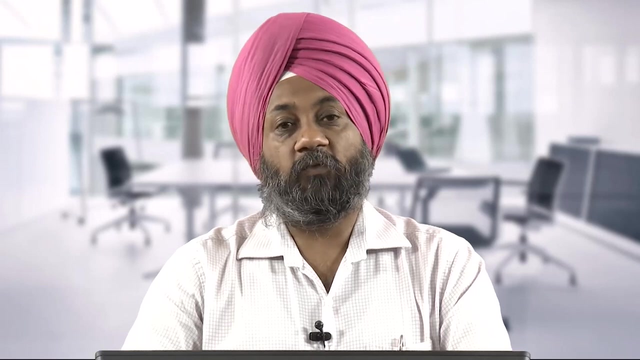 design to be successful, 3 important things are very, very important, or very, very, you can say, necessary. First thing is that we must be very, very careful while designing the product. So the first key word, or the catch word, is the design of the product. 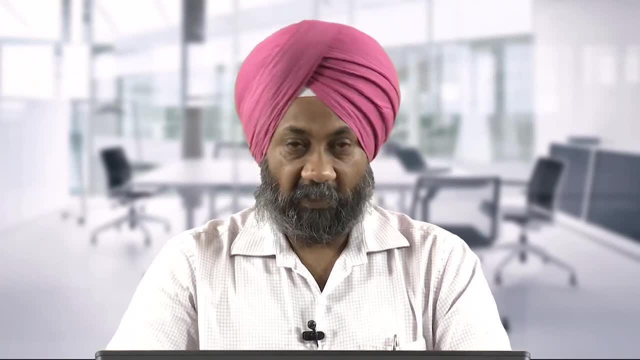 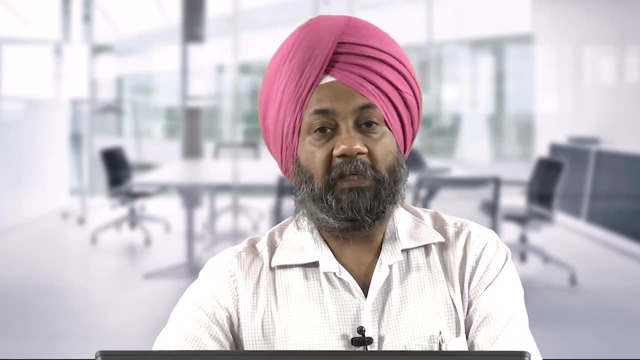 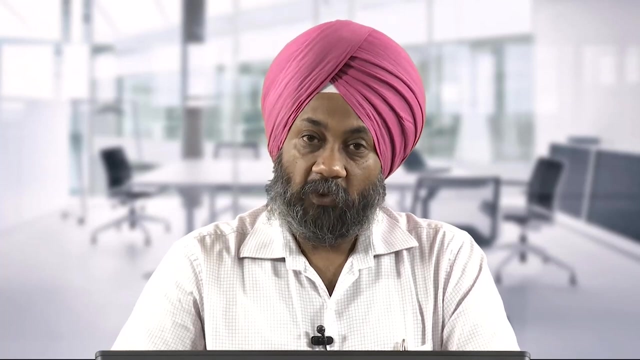 Now for design of the product. there are number of guidelines, there are number of steps that we have to follow. We have to ensure that the design is robust. the design is such that it satisfies the functional as well as the aesthetic requirements of the customer or the need for which the product 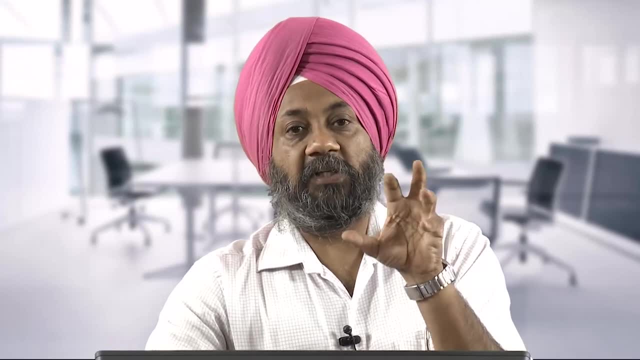 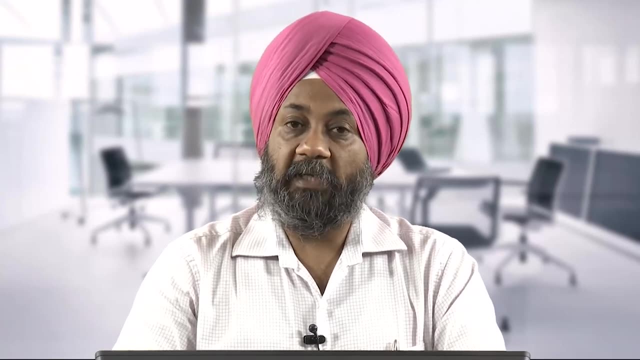 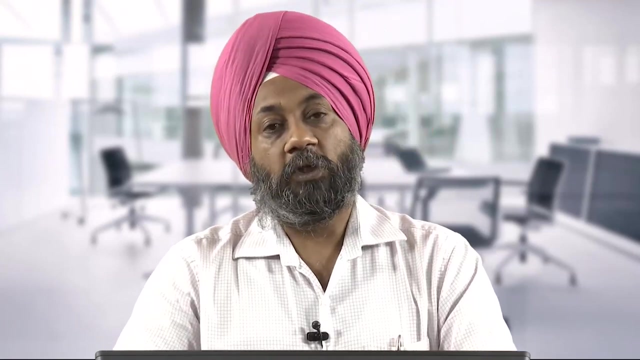 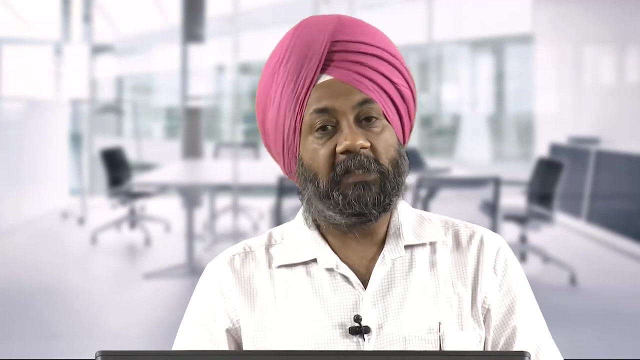 is being designed. So the first catch word is design. The second catch word is the materials that are going to be used for making that product and a third important thing is the manufacturing process that is going to be used for manufacturing that product. So these are the 3 important things. again I will highlight- and this we have already- 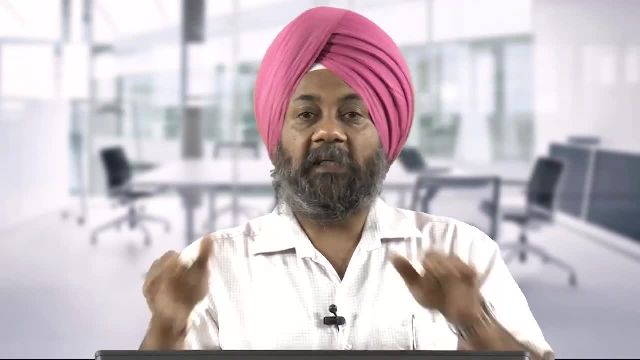 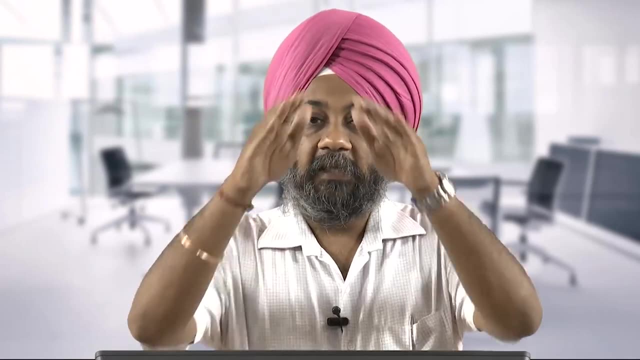 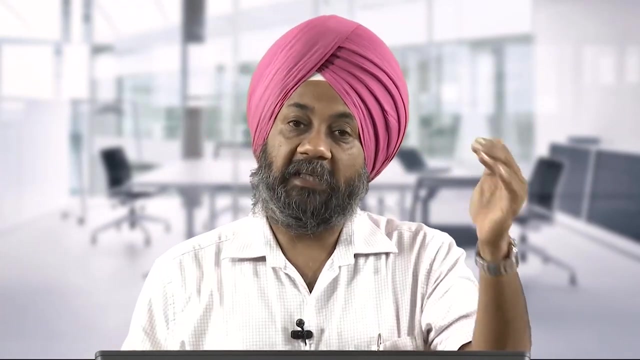 seen in our very first week of discussion That in a triangle identifying the quality of the product or defining the quality of any product, 3 important edges of the triangle or 3 important sides of the triangle play a very important role, and one side is the design. 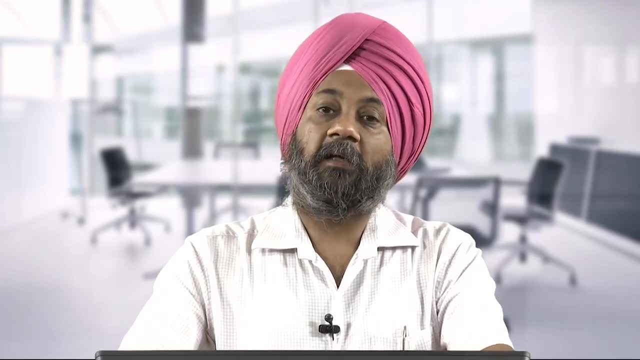 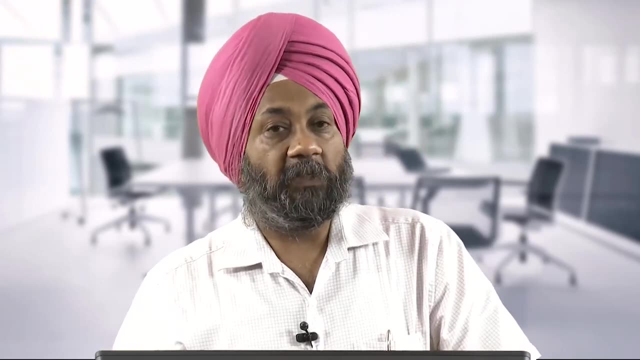 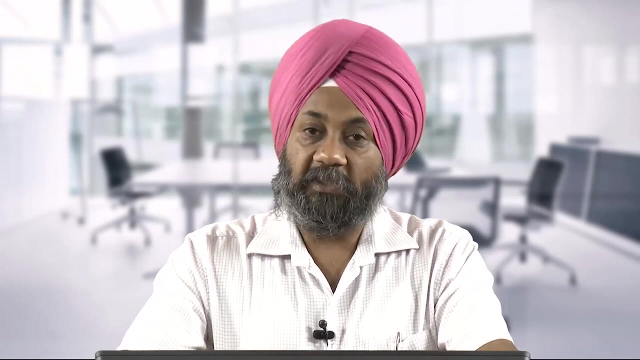 The second one is, as you are well aware, is the materials and the third one are the manufacturing processes. So the importance of materials cannot be sidelined or neglected from product design point of view. So we have to keep in mind the product design or the importance of materials in product. 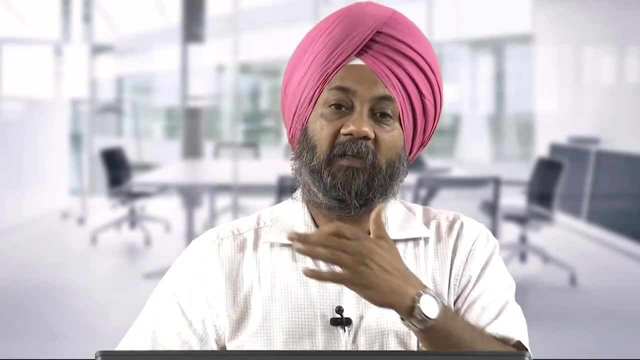 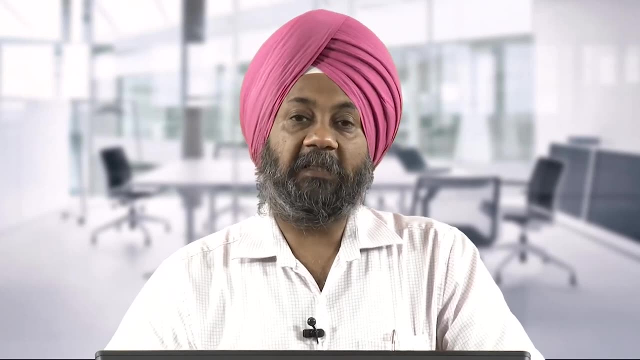 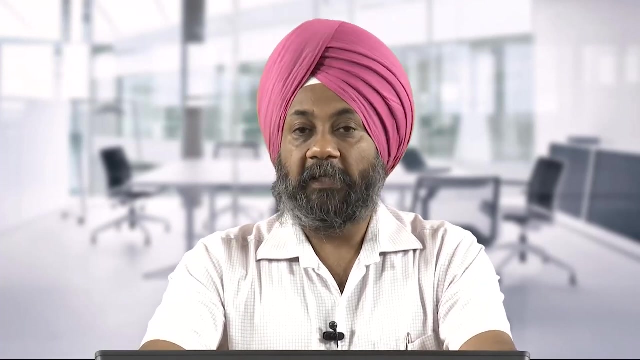 design. So today we are trying to see that there are a large variety of materials that are available with us, So we try to select the most optimal material that is going to satisfy our functional as well as the other service requirements for the product being designed. 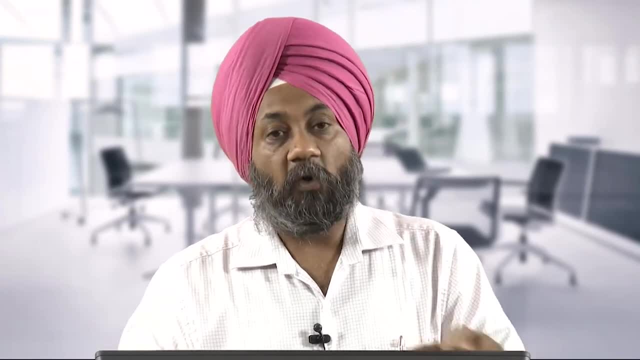 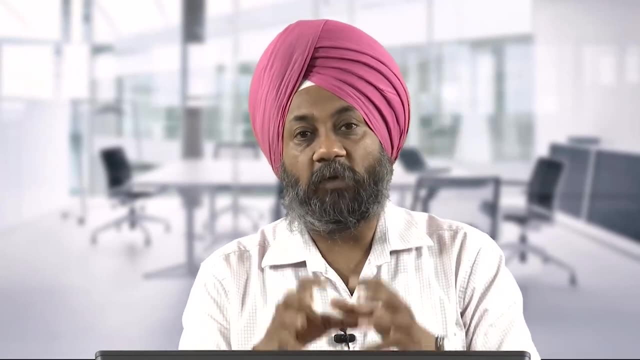 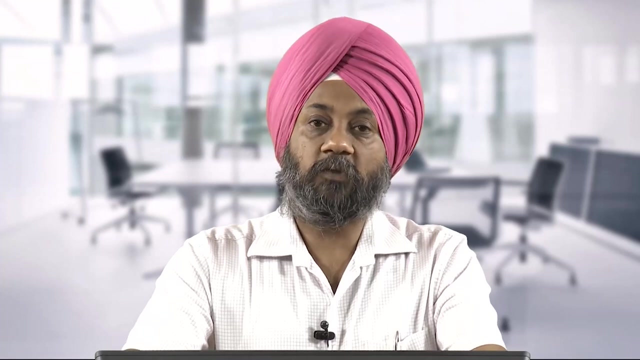 Now let us see that how we select a material. So how we select a material, that we will study in selection of materials 2 and in selection of materials 1. we will see that what are the parameters governing the selection process of engineering materials for different types of products. 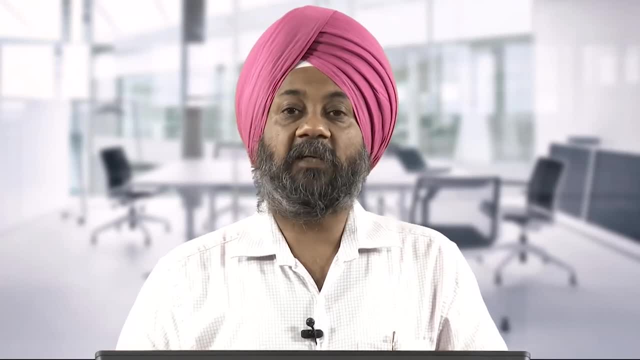 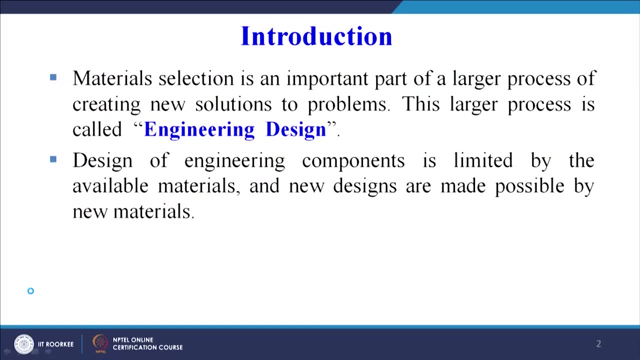 So what can be the various guidelines that we will try to understand. So the materials selection is an important part of a larger process of creating new solutions to problem. So we try to find out new solutions to the problems and it is an important part. 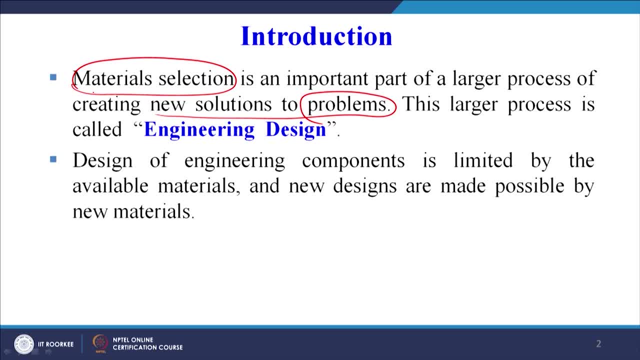 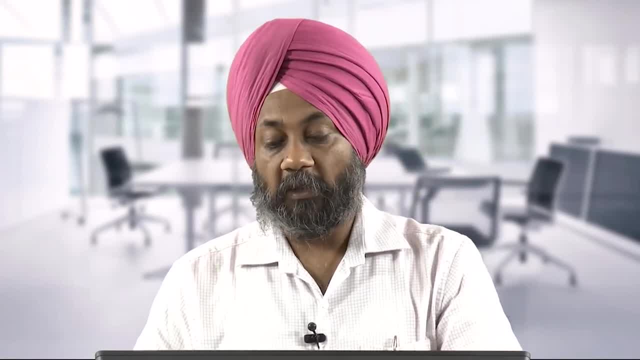 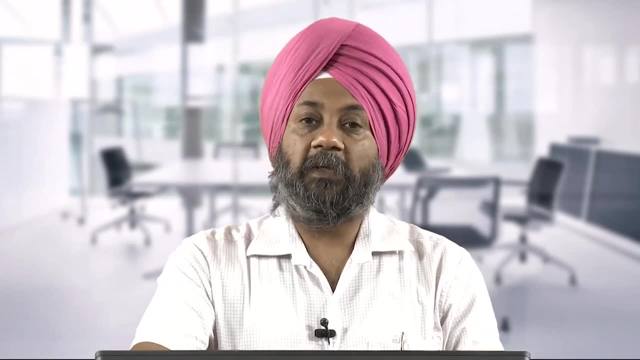 Materials selection is an important part in our problem solving approach or in our problem solving endeavour. So the material selection is an important part of a larger process of creating new solutions to problems. Now we can take an example again of maybe furniture. Let us see. 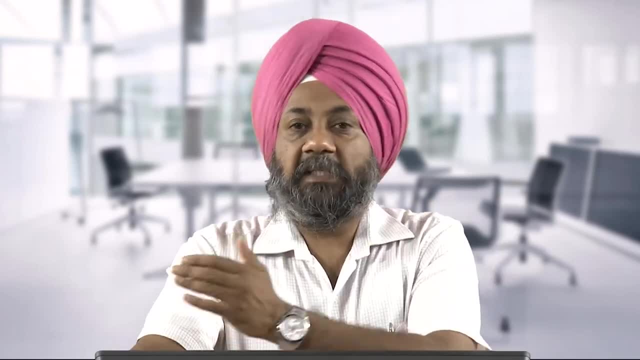 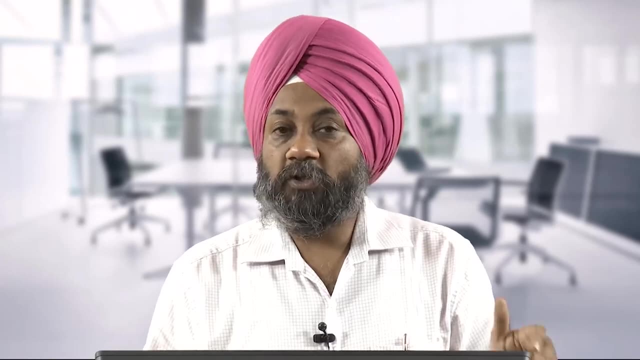 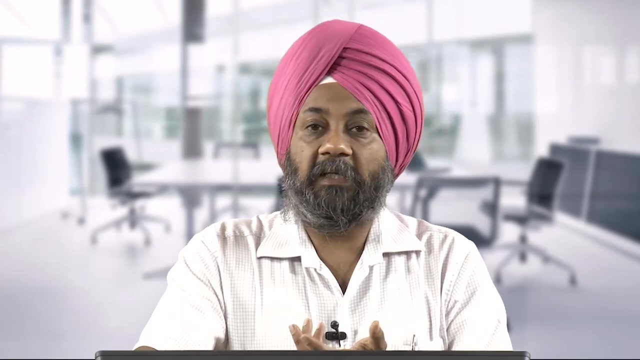 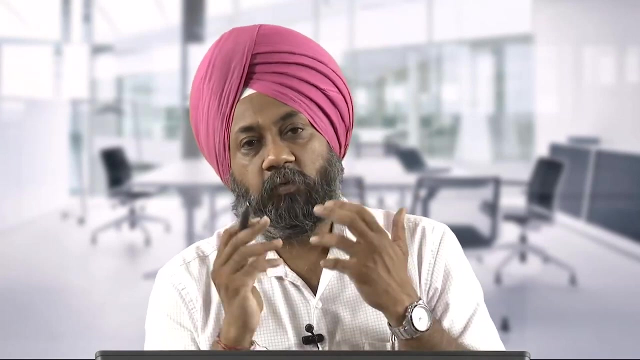 We are seeing for so many years. the design of furniture is changing day by day. Why it is changing? because new and new materials are being invented. So when new materials are available with the designer, he can experiment, he can try to see, he can try to visualize his design in a different manner, because now he or she feels 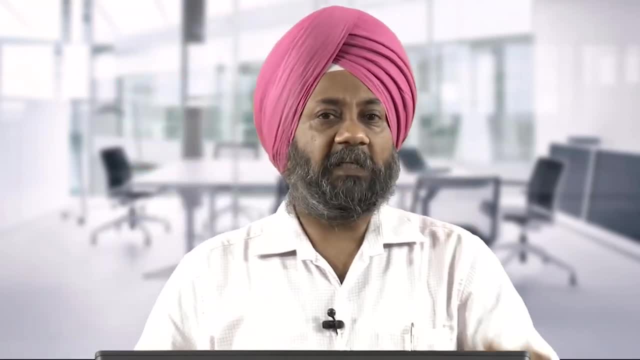 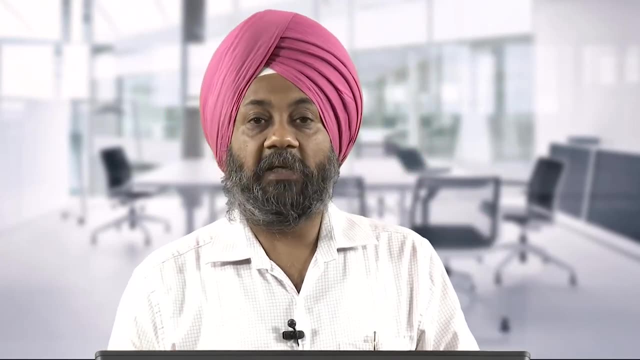 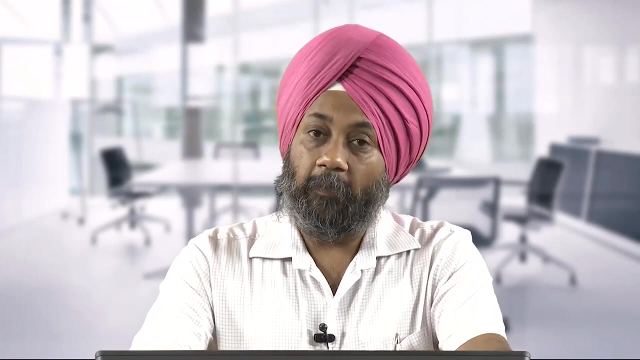 that, yes, this extra or this additional, This additional material is available with me, and if we can use this material for making our furniture design, or making a sofa set, or for making a chair, or for making a table, definitely new designs will come up. why? because now, new materials. 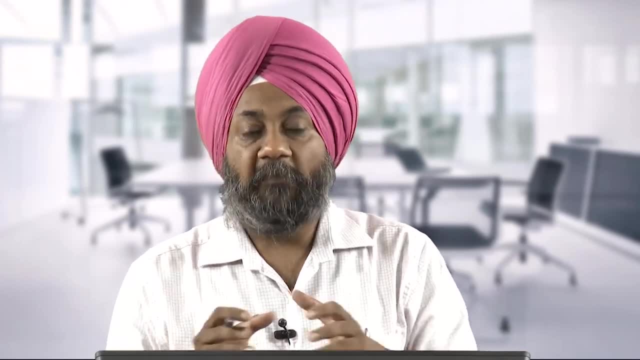 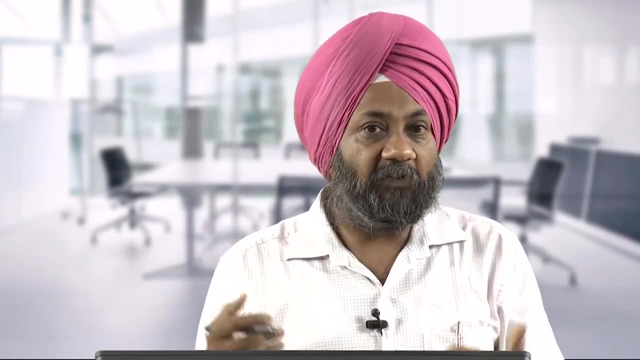 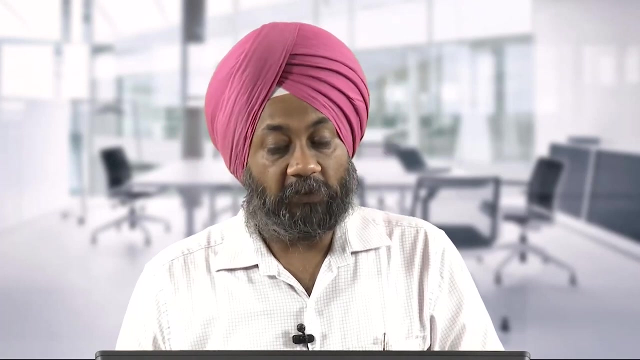 So the library of materials has increased, or the family of materials may have new members, So these new members may help the designers to think more creatively and coming up with the shapes which were not initially possible with the available materials. So that is the important point in the first sentence, that is, materials selection is an 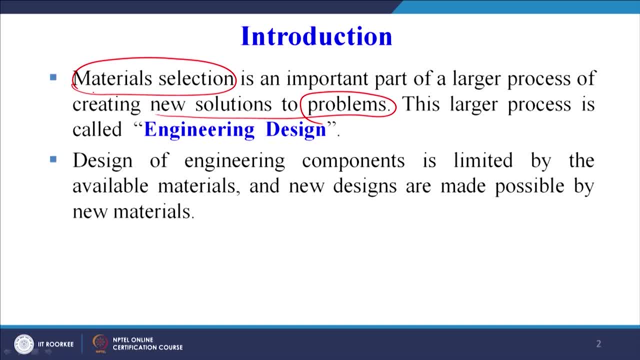 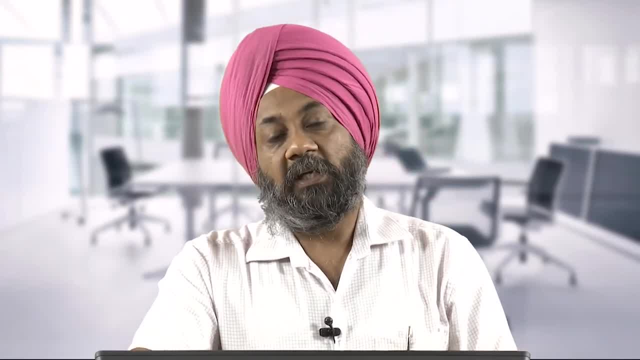 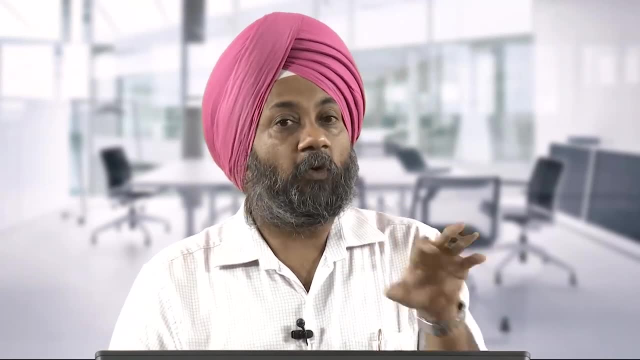 important part of a larger process of creating new solutions. So new solutions will definitely involve creativity, it will involve design thinking, it will involve the step by step procedure for finding out the solution. but we cannot ignore the importance of materials in this larger picture. 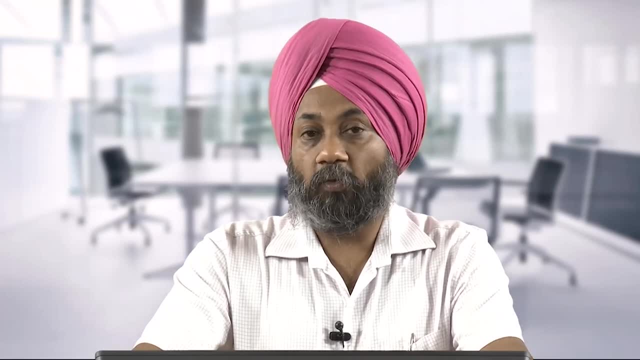 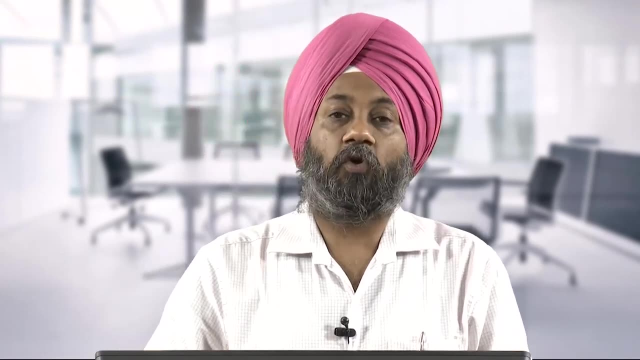 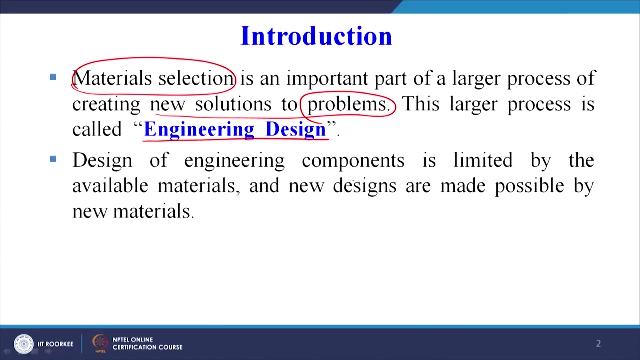 In this larger picture. materials will also play an important role in defining the final product or the design of the final product. This larger process is called engineering design. So when we talk of engineering design, we cannot ignore the importance of engineering materials. So it means that engineering design will also require knowledge of the materials. 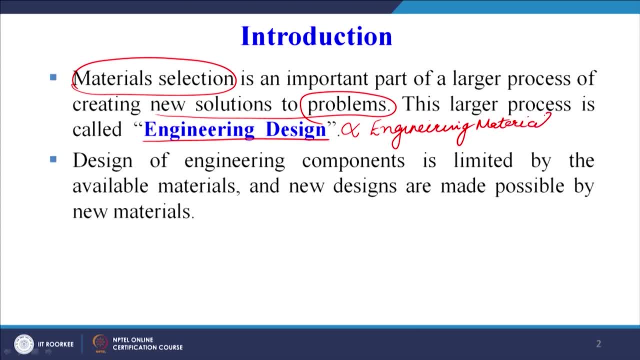 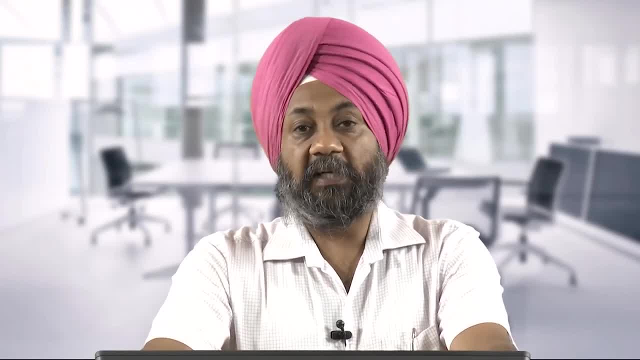 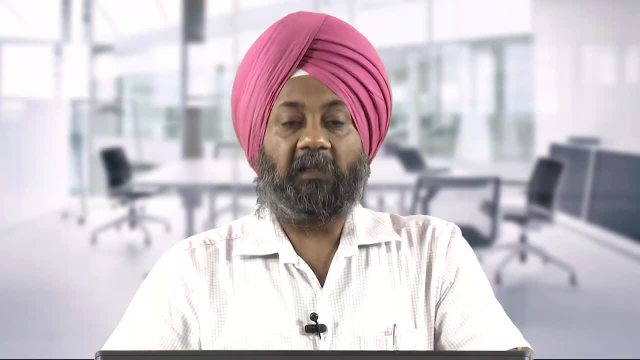 Engineering materials and therefore we are discussing this topic- that why engineering materials are important and what are the factors governing the selection of the engineering materials. So design of engineering components is limited by the available materials. So this is very, very important sentence. if we are able to understand this sentence, we 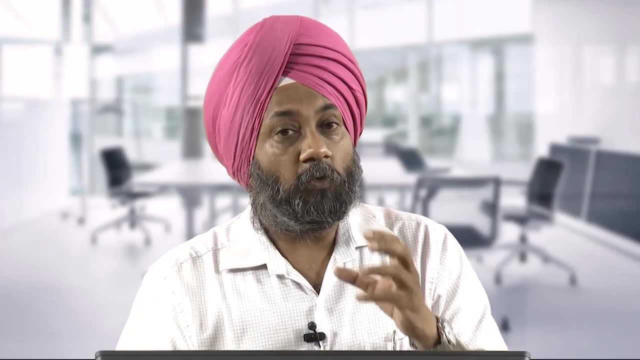 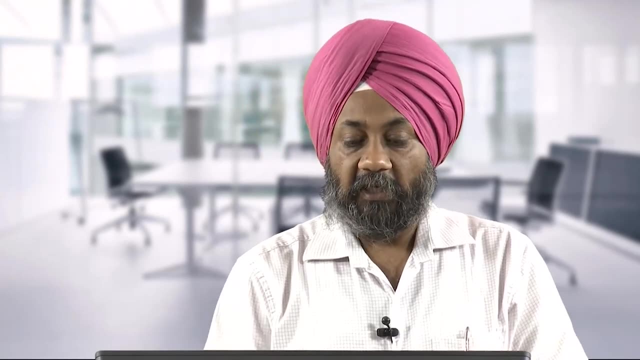 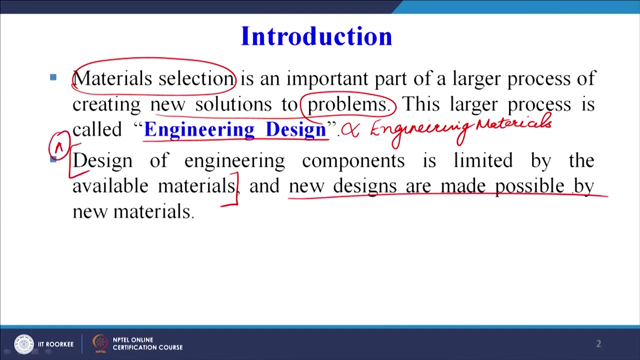 will be able to emphasize. We will be able to highlight the importance of materials. We will be able to highlight the importance of materials in product design. So you can just try to break this sentence into 2 broad categories: this is A and this is B. 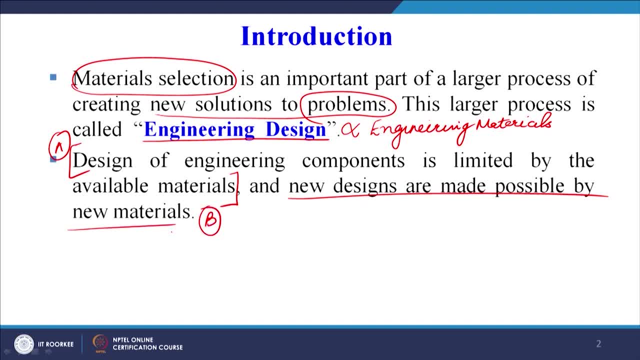 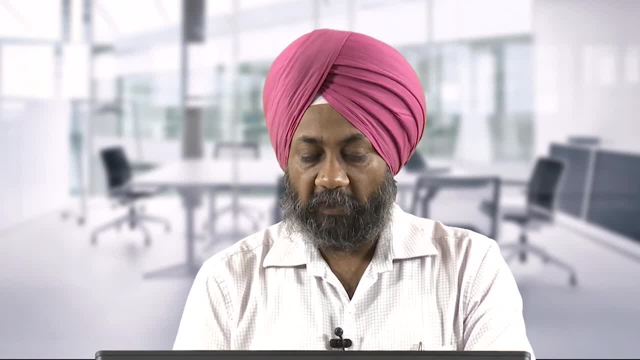 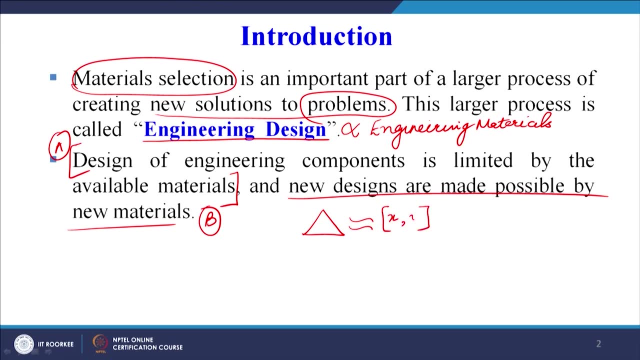 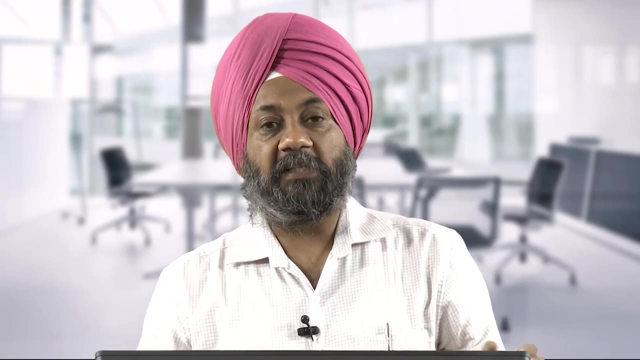 So if you look at A, what is happening in A design of engineering components is limited by the available material. So suppose we have a design of a product and we have to choose a material. we have limited set of materials, that is X and Y. So we have a design and we have available set of material, so this design is limited. 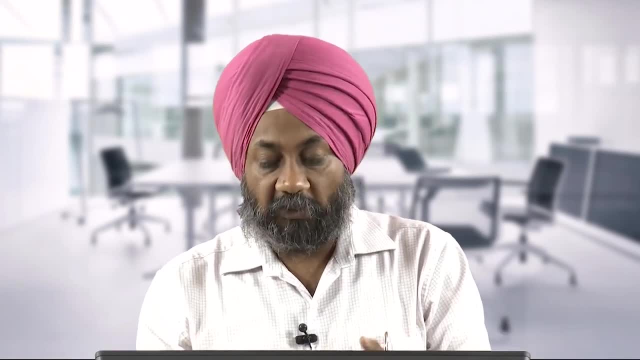 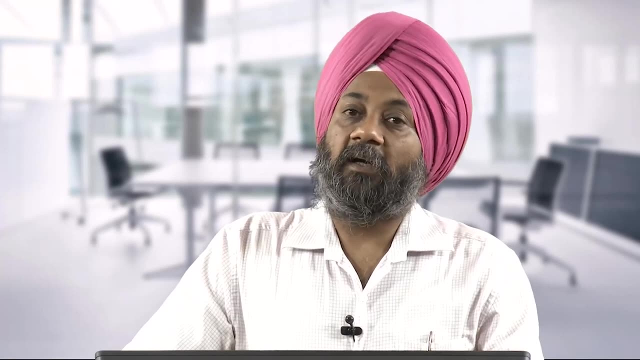 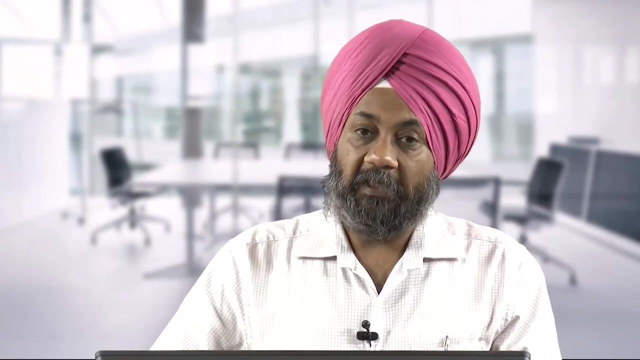 by the available set Y, because we can make this design with these 2 materials only and there is no additional modifications in the product design possible because we have available materials only. But if we come to B, new designs are made possible by new materials. now suppose you want to change. 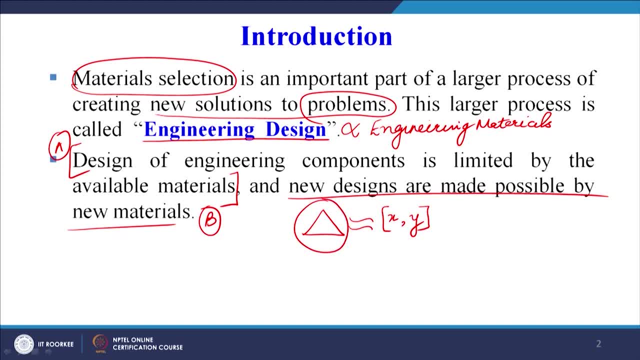 the shape Of this product. it was limited by the choice of materials that we have. but now we say we have different types of materials which are available with us. Now we can experiment with this shape of our product or component. why? because now we have additional materials. we have 4 additional materials which are available with us. 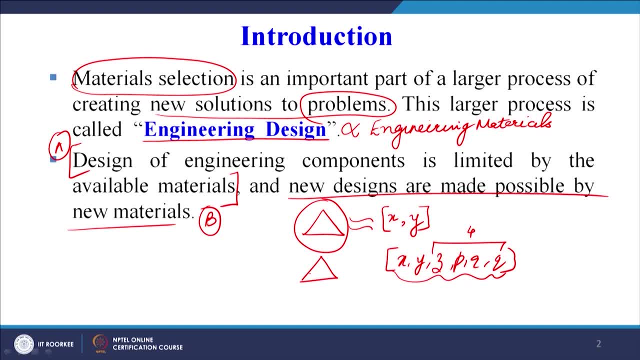 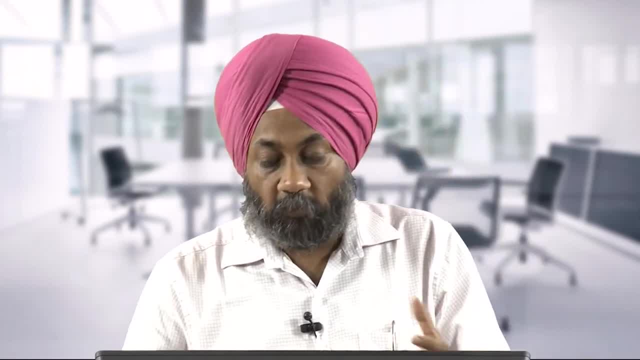 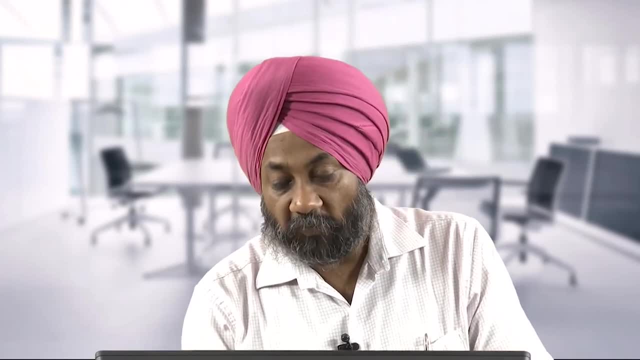 So they are. definitely we can experiment with the shape Of the product, with the size of the product, with the functionality of the product, with the aesthetic of the product. why? because now we have large variety of materials that are available with us. But the problem is now, if we have a large variety, how to choose, or what is the criteria. 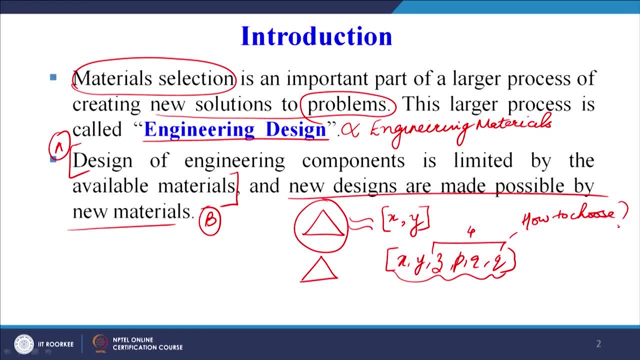 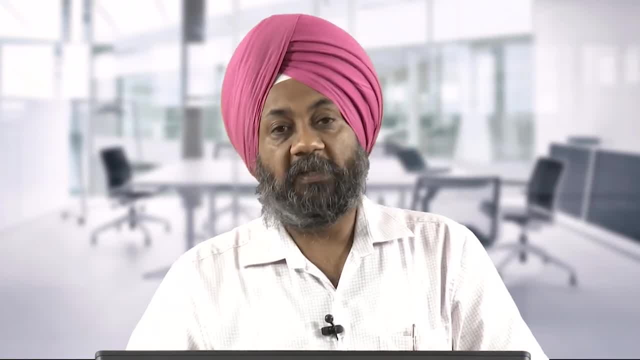 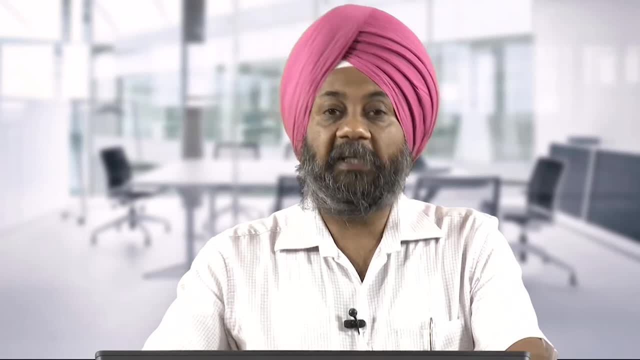 that we must follow to select a material out of these materials, And I think this we have already discussed with the help of a chair in one of our previous sessions. so these are the 2. we can say guidelines or guiding factors when we talk of materials. 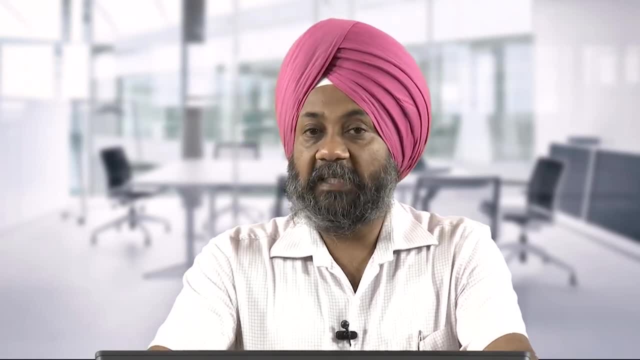 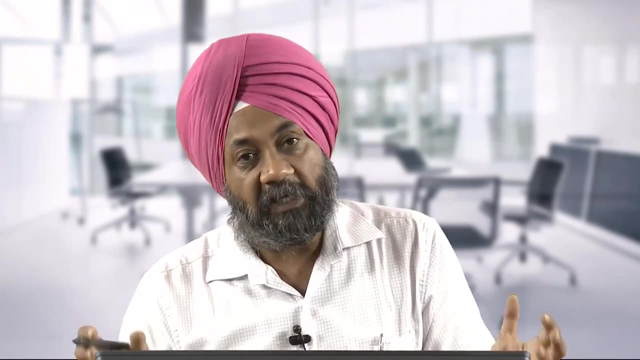 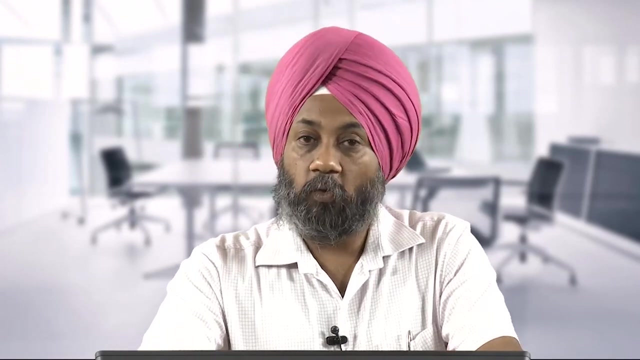 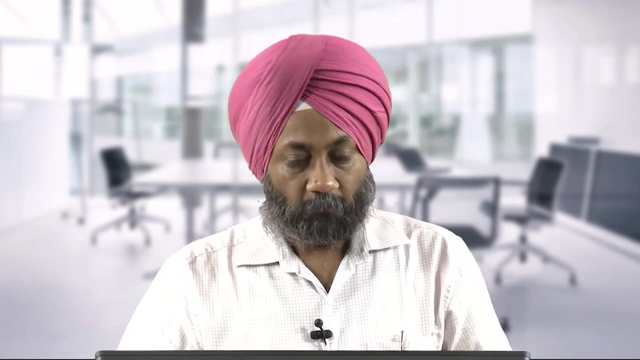 representation or importance of materials in context of product design. So limited materials. we have limitations in term of product design. a wide variety of materials: we have a choice to design our product accordingly, but then there is a problem that how to choose the best material for the product, and for that we are trying to discuss today. 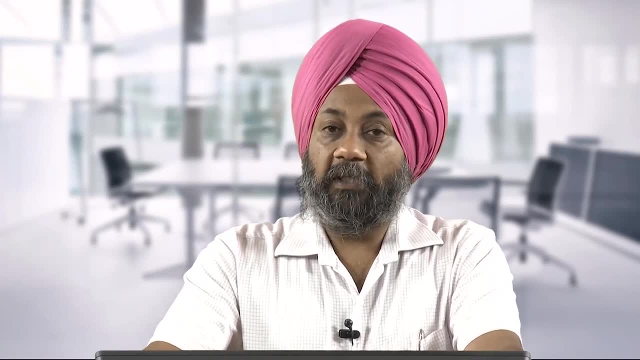 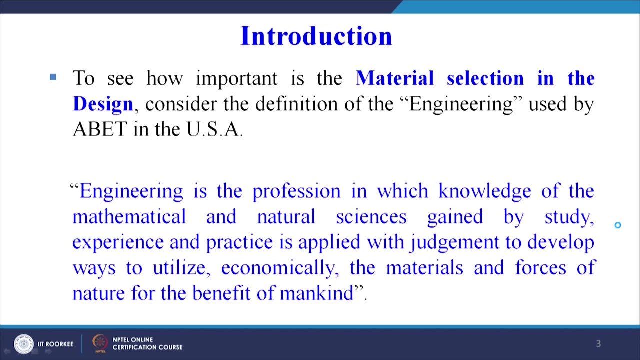 Now, material selection is important. another important definition of engineering that is there on your screen: this is material selection in the design. So the definition of engineering says: now: this is according to the accreditation board of engineering and technology in the USA, so we can see this definition. this is very 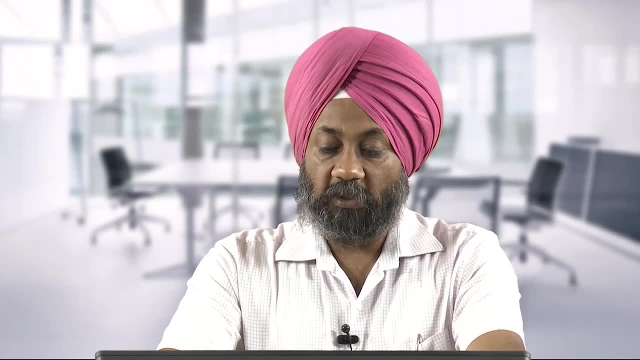 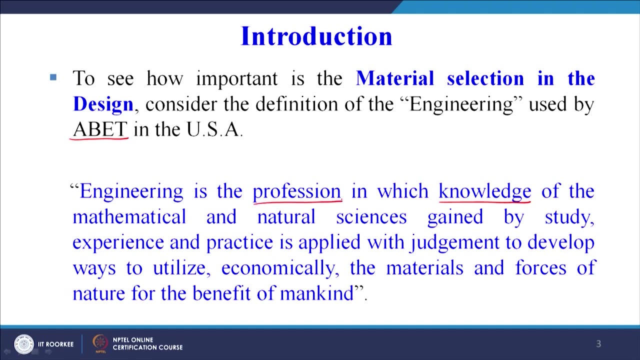 very important. Engineering is the profession in which knowledge of the mathematical and natural sciences. so in this profession we use the knowledge of the mathematical and natural sciences which is gained by. how do we get this knowledge? by study, by experience and practice. This is applied with judgment to develop ways to utilize economically the mathematical and 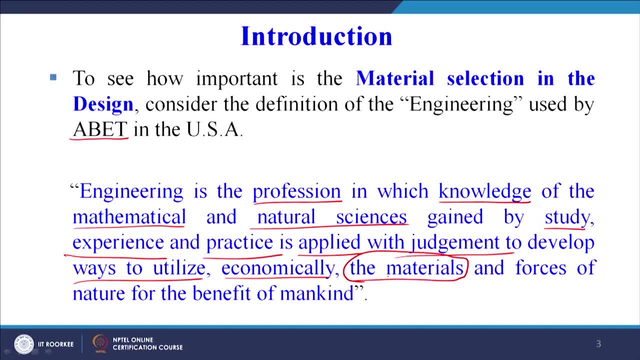 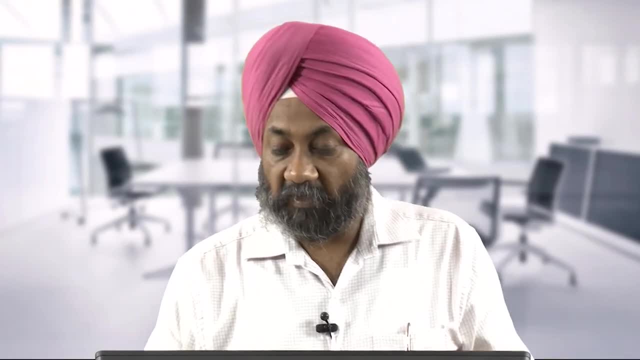 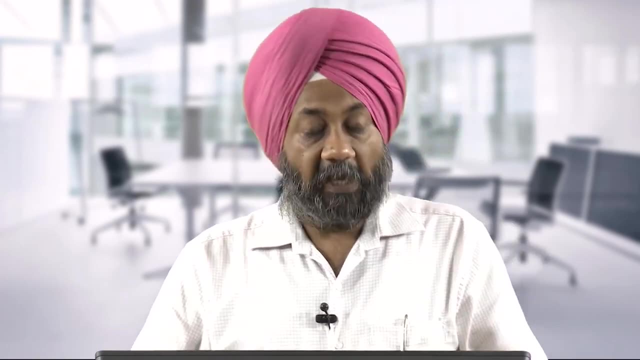 the natural sciences. now, how we have gained this knowledge. we have gained this knowledge by study, by experience, by practice, And then we try to apply this knowledge to economically use the materials and forces of nature for the benefit of man. Okay, 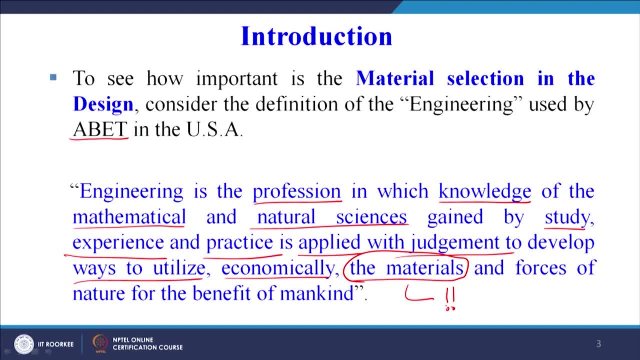 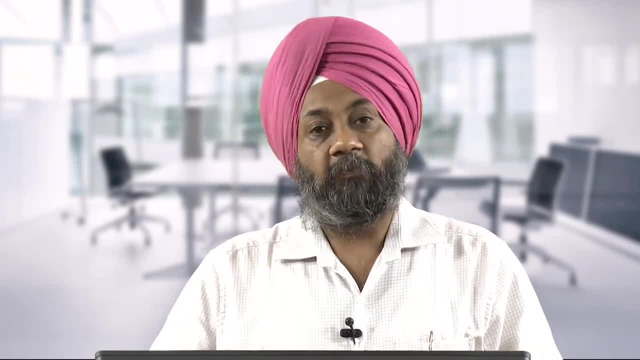 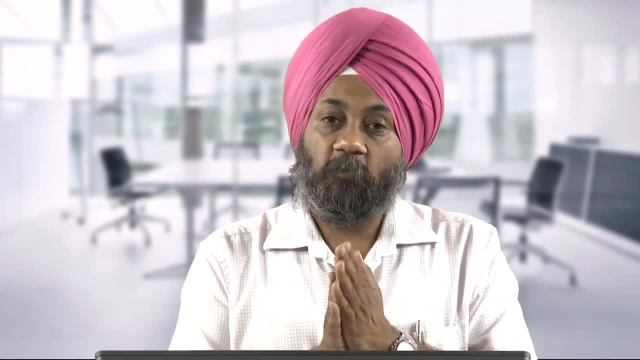 Mankind. so we try to develop tangible products which are going to affect the mankind or which are going to make the life of people easy. life of people may be happy. So therefore, the materials are also an important aspect in any engineering design which cannot. 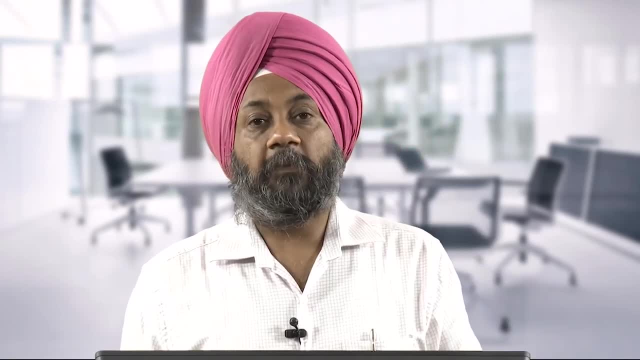 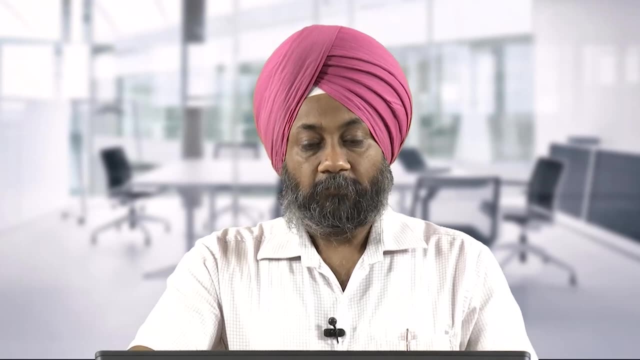 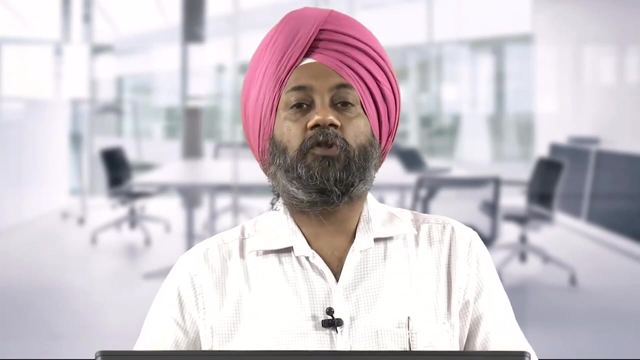 be ignored. So we have to highlight the importance of engineering materials, and it is also highlighted in the definition of engineering. Okay, Now let us see the need of material selection. already we have now, I think, amply addressed this point, that what is the importance of engineering materials? 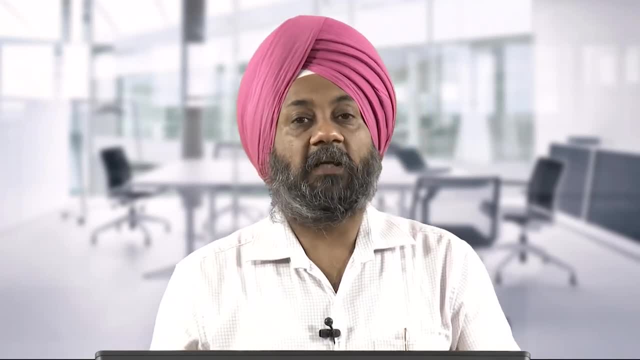 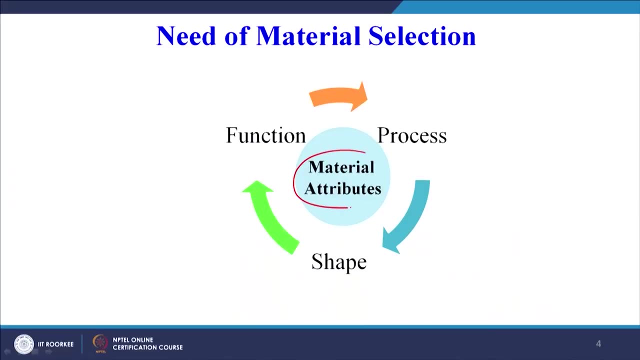 Now let us try to see that. what are the factors that will govern the selection of materials? Now, material attributes are very, very important, and how they are important because they will define the function, Okay, The process which is going to be used for making the product, as well as the shape of 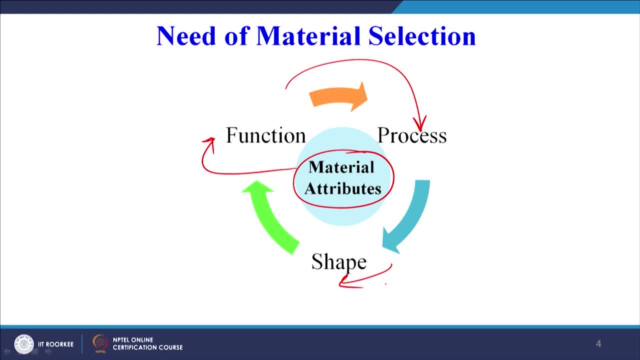 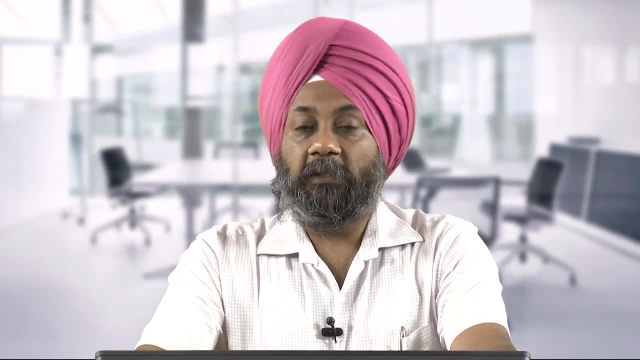 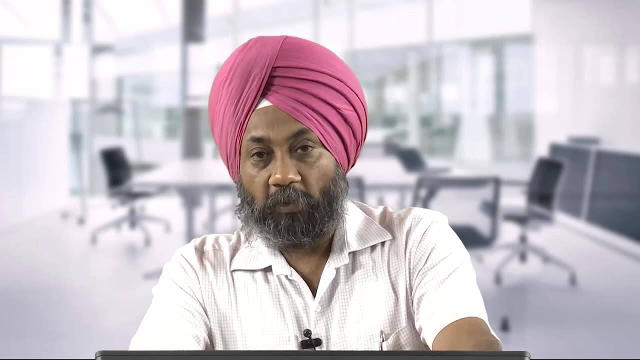 the product. So the need of material selection is important because it will further lead to the decisions related to the functionality of the product, the process that is going to be used for making the product, as well as the shape that can be given to the product. 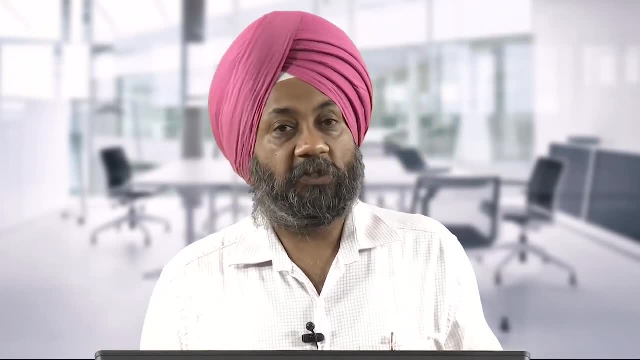 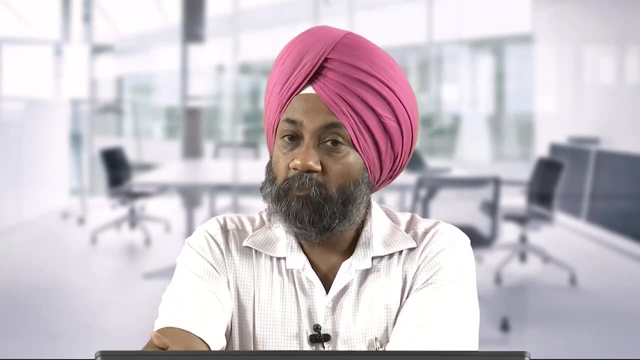 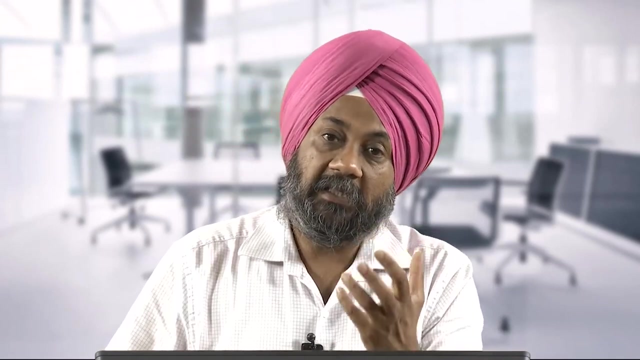 Now, if you remember, in our first week of discussion we talked about the basics of manufacturing. Okay, The basics of manufacturing processes, and shape was an important criteria there. So different processes can make different types of shapes. similarly, we can say different materials can take different types of shape. there can be materials which are which we 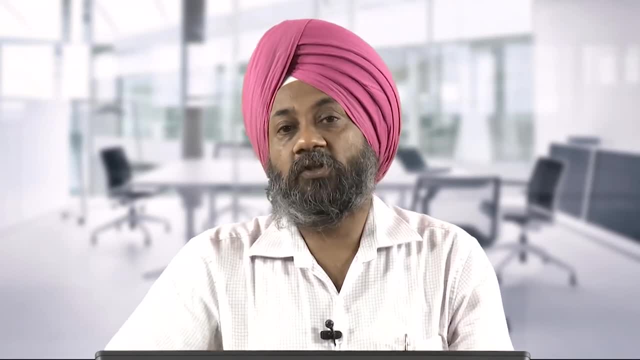 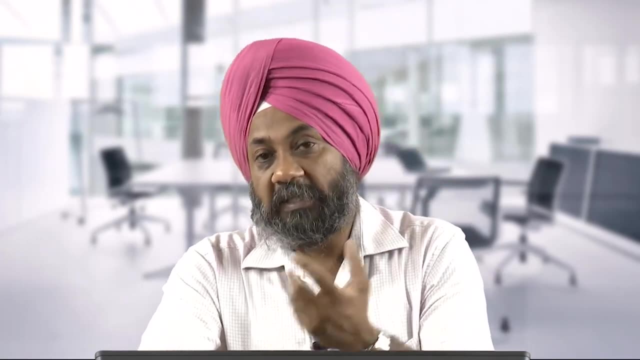 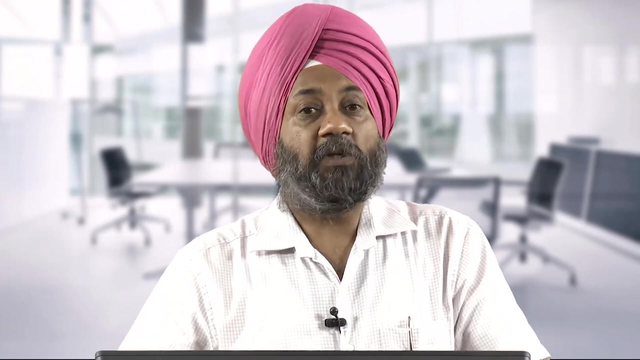 may not be able to give a very, very complicated shape, even with the most advanced manufacturing process. So, shape, functionality, the process that is going to be used- Okay, That is completely going to be dependent upon the material attributes. So we need to have a basic understanding about the engineering materials. 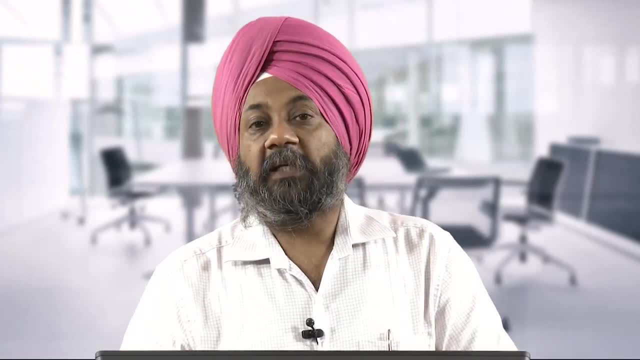 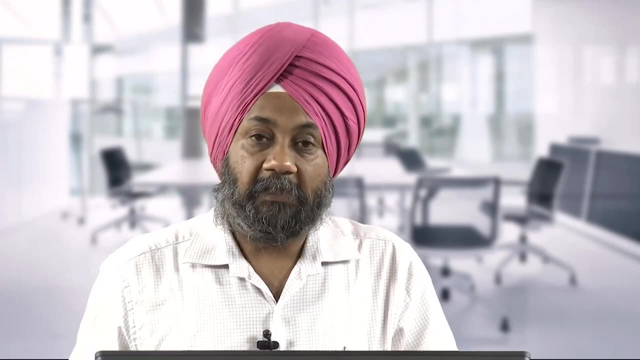 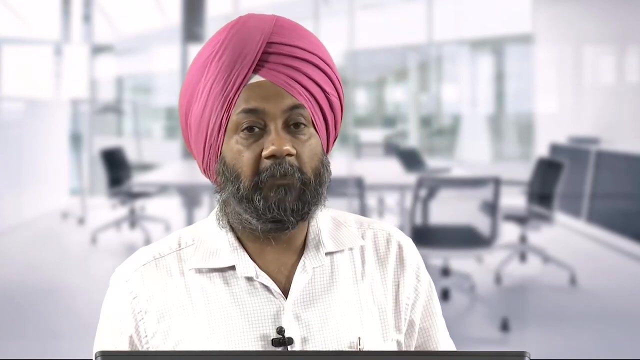 We have already discussed, if you remember, the classification of engineering materials, and then we have taken the basic characteristics of the different materials. But we have 20 hours of discussion with us, So we are going to discuss 2 and a half hours on engineering materials, which I believe is. 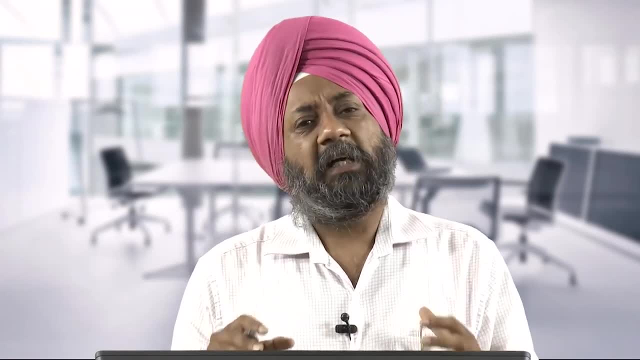 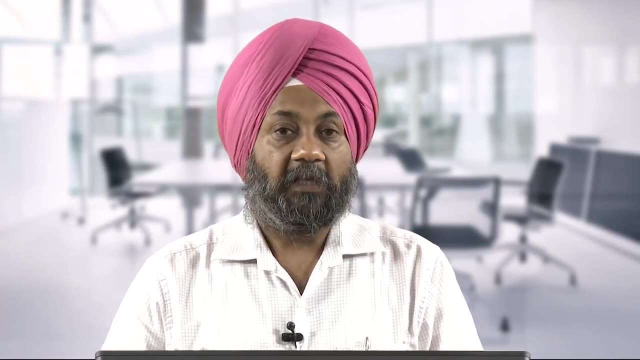 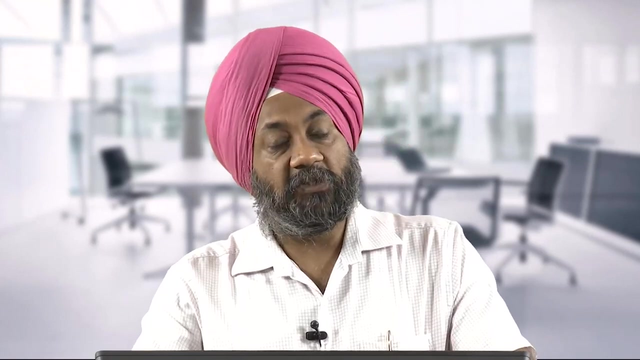 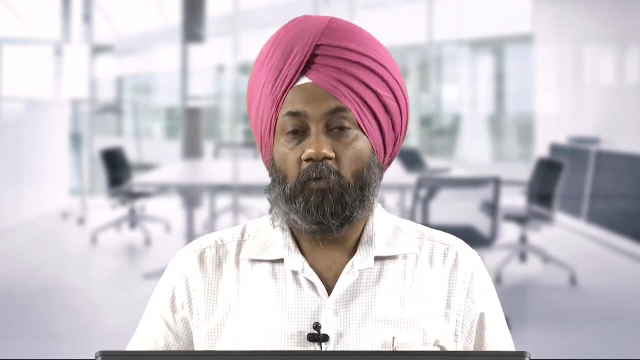 not adequate time to properly understand the concept of materials. But why we have included it is that, as a product designer, every designer must have a basic idea about the materials, Because if that basic idea is missing, the design that the designer proposes may be sent back from the manufacturing department. why? because it may not be feasible to produce. 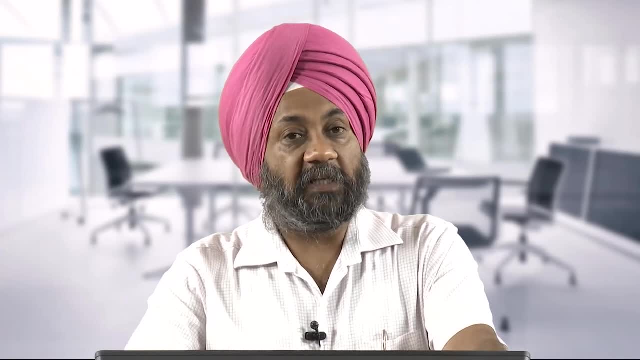 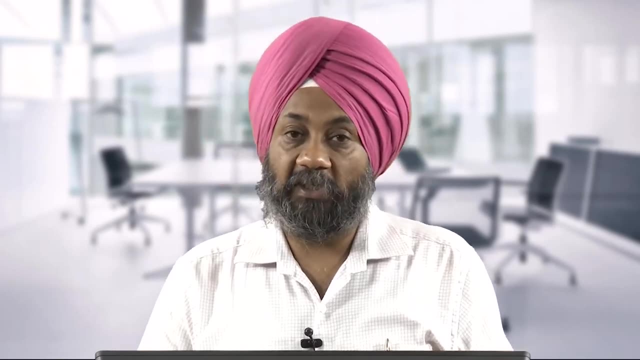 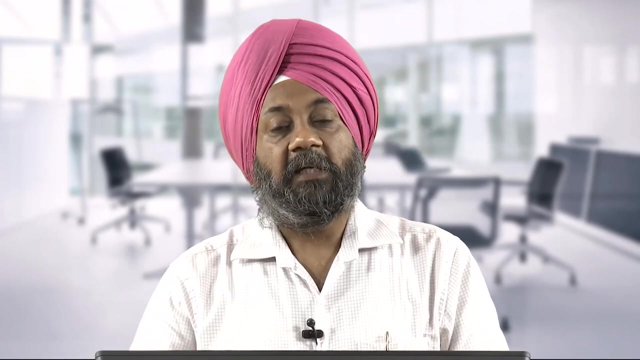 that product. So we need to have a basic understanding, as per the material suggested by the designer or as per the manufacturing process suggested by the designer. And therefore, in order to avoid that iteration, or to avoid that review of the design, or to avoid that reworking of that design, it is better that we have fundamental understanding. 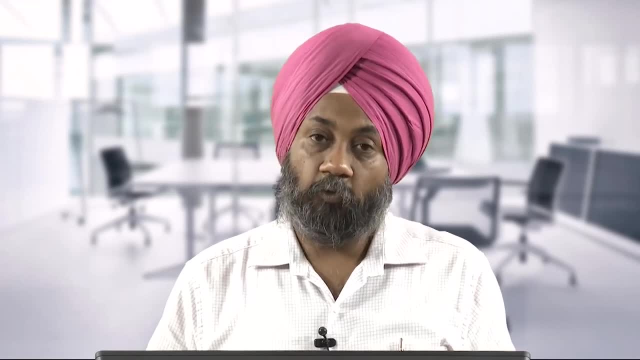 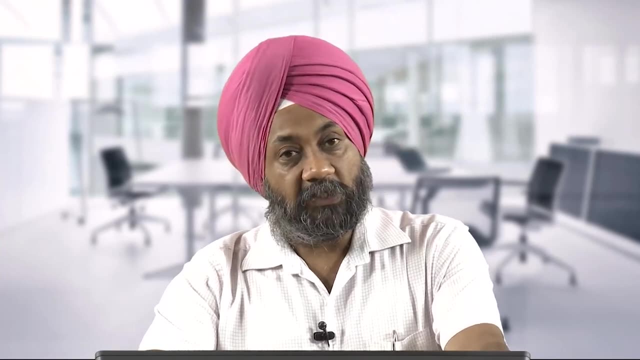 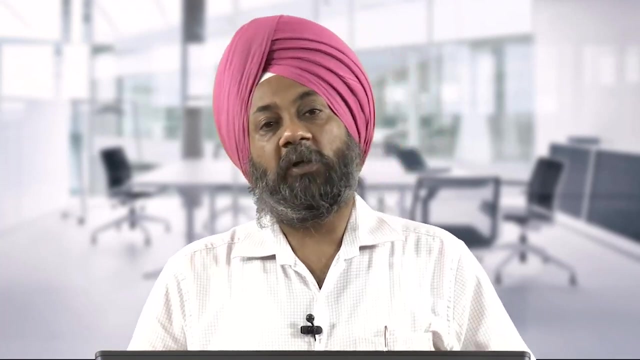 of the materials as well as the processes, before passing on the final design to for manufacturing or to the manufacturing team. And in these days such situations are rare. why? because the product development team has experts from manufacturing, also from marketing, also from legal cell, also from copyright. 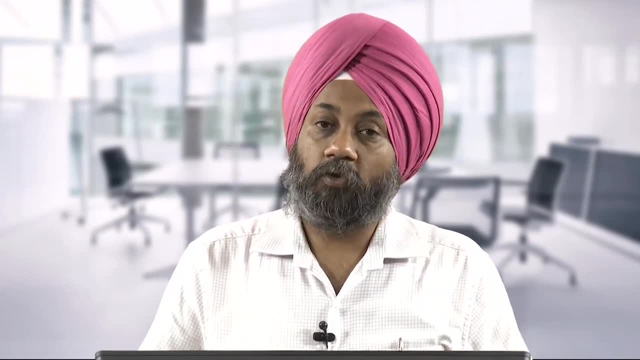 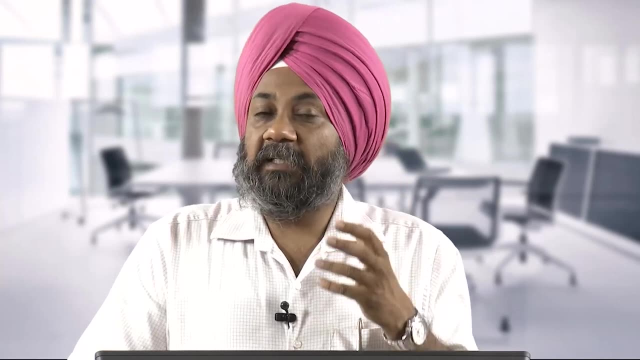 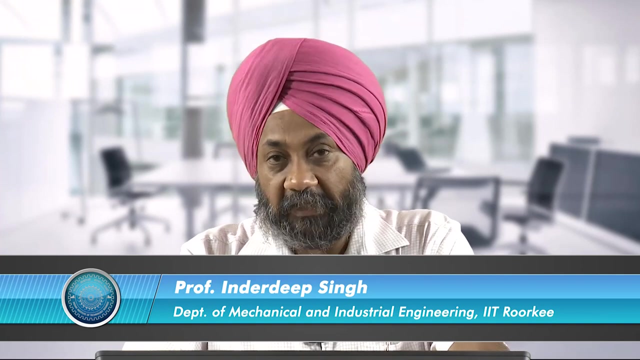 protection or IPR related lawyers also are in the product development team. So therefore all these things are taken care of. But when a designer is sitting and he is conceptualizing an idea, he must have basic understanding of that. So these materials, the processes and therefore this, there is an importance to study this. 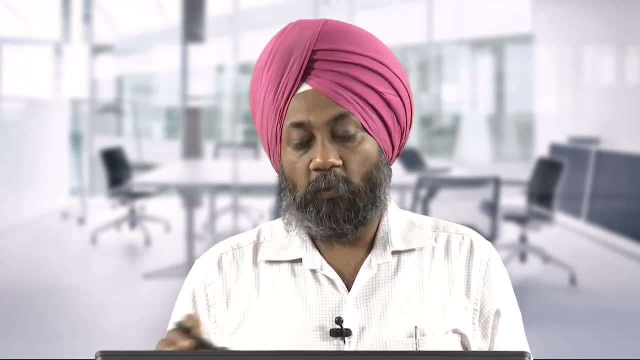 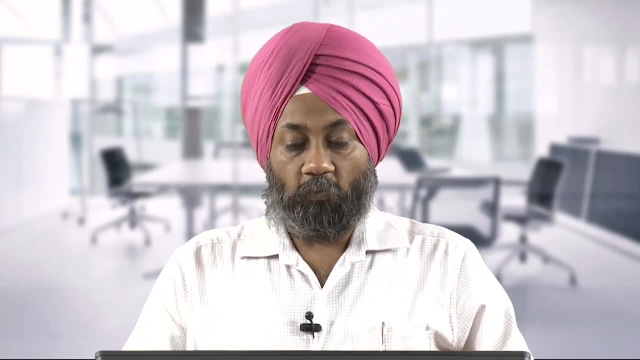 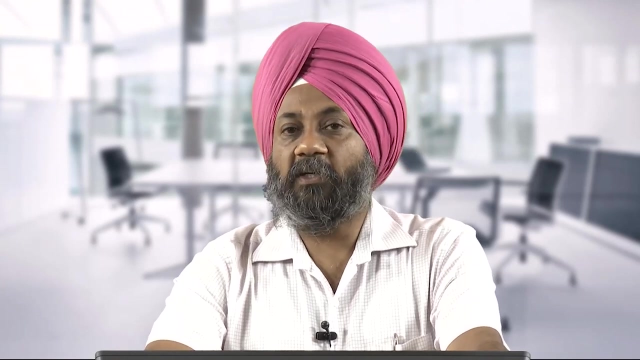 course. So these material attributes are going to affect the functionality, the process, as well as the shape that we can give to our product. Now what is the challenge in selection? We have understood now completely that engineering materials play a pivotal role in the product design process. 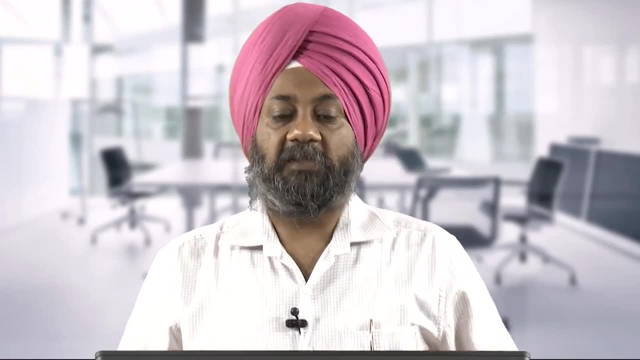 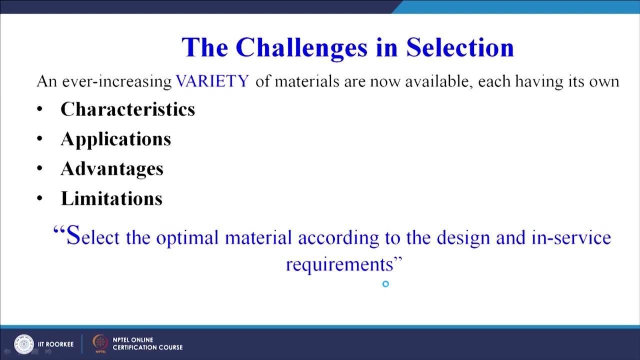 Now there is a wide variety of materials available with us. It is given in the verification. I have a sentence on this slide. The ever increasing variety of materials are now available, each having its own. each material. if you see a variety. What is the variety? if we talk of variety, we have, if you remember, metals, alloys, polymers. 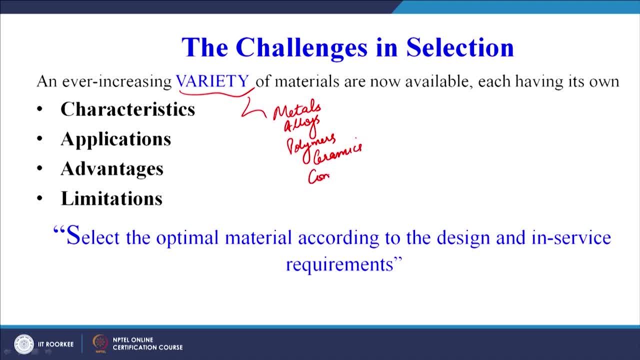 ceramics, composites, And how much? 25.5.. So what is the difference? And a lot of other families of materials. so we see just 5 families here, but there are other families as well. So we can see that we have a large variety and out of this variety we have to choose. 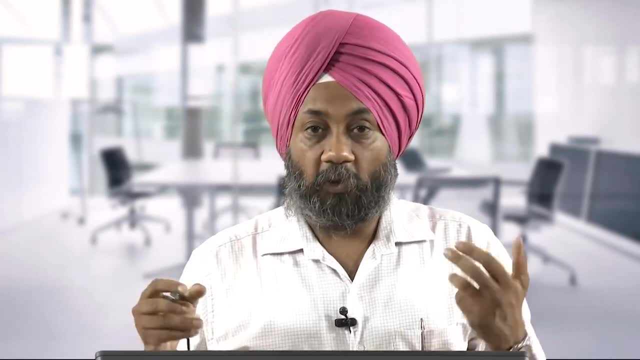 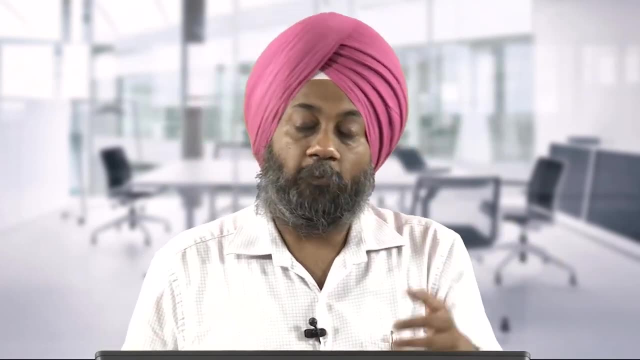 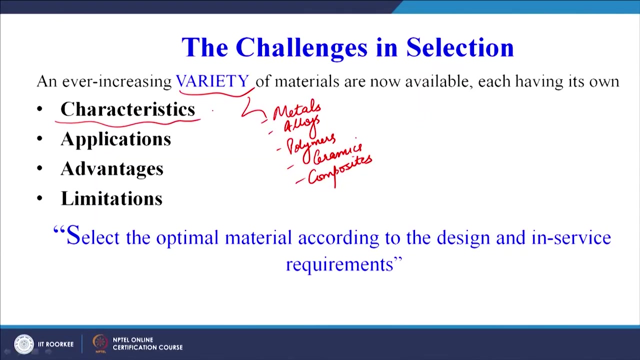 that which one is going to be the material of choice for my product design, whether I am going to make it in plastic, or I am to propose this product design in metal, or I am going to propose this product design in a ceramic. Now, that will depend upon the characteristics of the materials, that will depend upon the 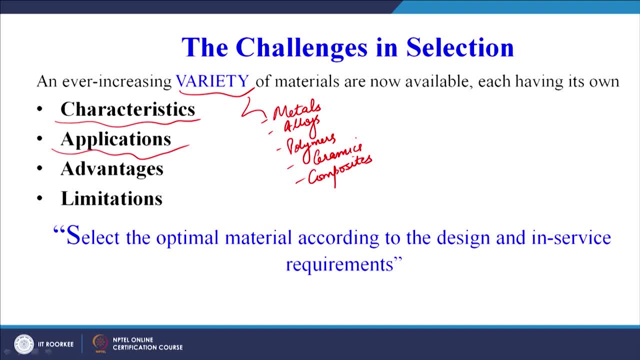 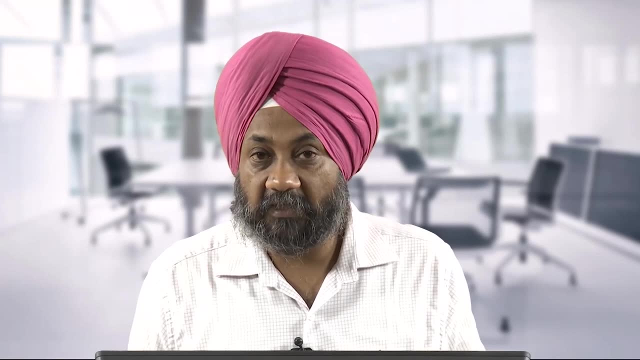 applications that are possible with that material. and this application and advantages will depend upon the properties of the material, which we have already covered. If I ask you just, I may give you 10 seconds to just remember what are the various properties of engineering materials. We have already taken one lecture of half an hour on that, which was not a very exhaustive. 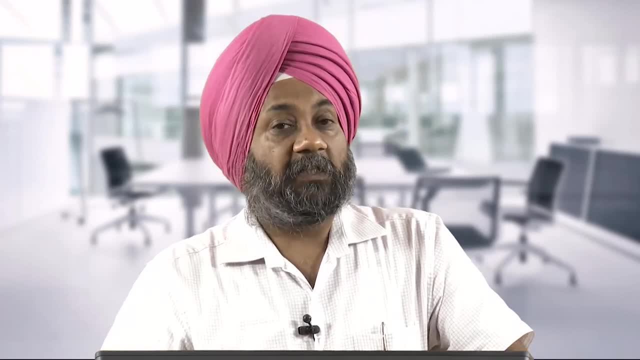 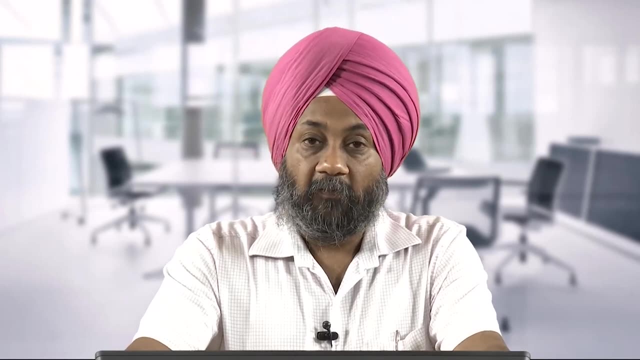 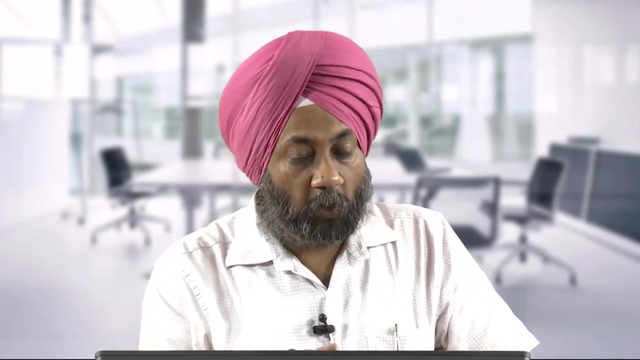 lecture. Still, we were able to understand that what are the important properties of engineering materials? and we have seen that there are physical properties, chemical properties, as well as we have seen physical, chemical, mechanical properties, thermal properties. So all those properties will define the applications. those will define the advantages and limitations. 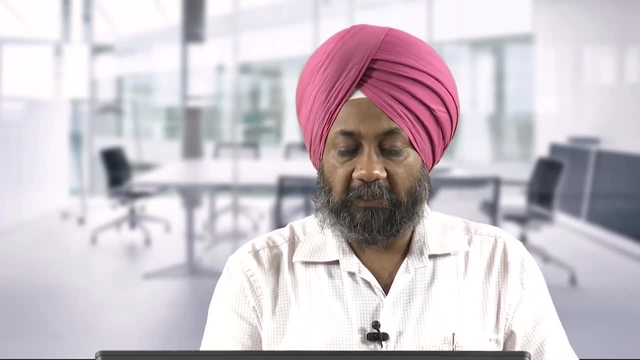 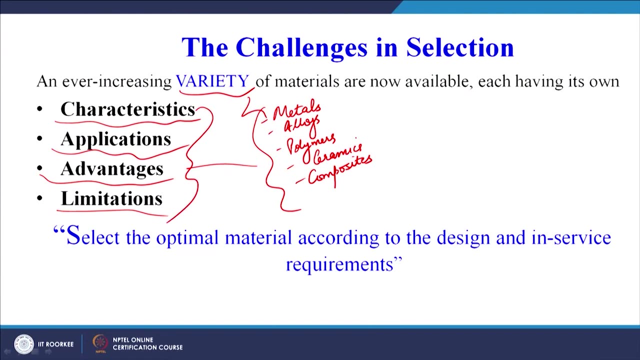 of the materials, So each of these materials will have their characteristics. Now we have to see that which one out of this we must choose for our product design. Suppose we say that we are going to use a polymer, so it is going to be a plastic product. 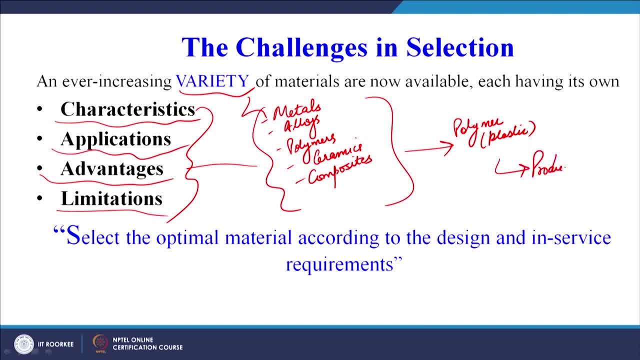 that I am going to make. So how to choose this process or how to choose the material. so we have a long list. we have to choose one. We have taken the decision. this answer we have to our problem, but how to choose that. 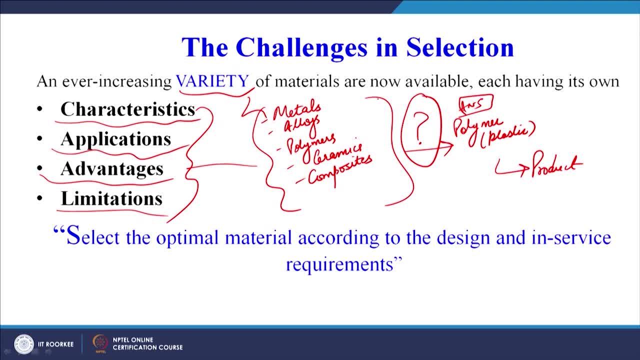 is one important point that we must all understand as product designers. So therefore, we need to select the optimal material. Now, this optimality is a big question mark. we have to select the optimal material according to the design, So this is one guiding factor here. 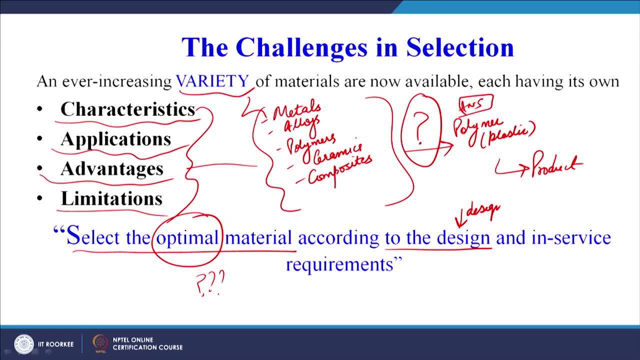 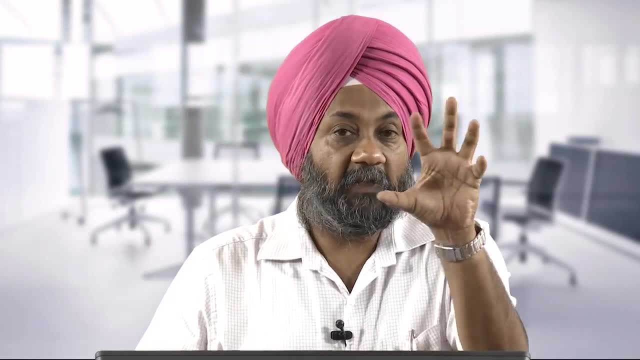 We have to see the design and second thing, we have to see the in-service requirements. So first thing is we have to focus on our design, as I have already told you in the very beginning in today's session, where we have taken that we have a design. 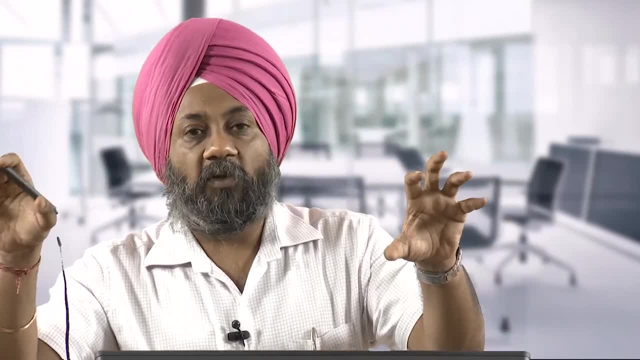 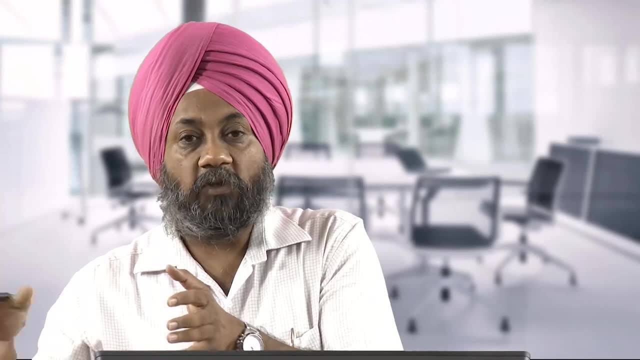 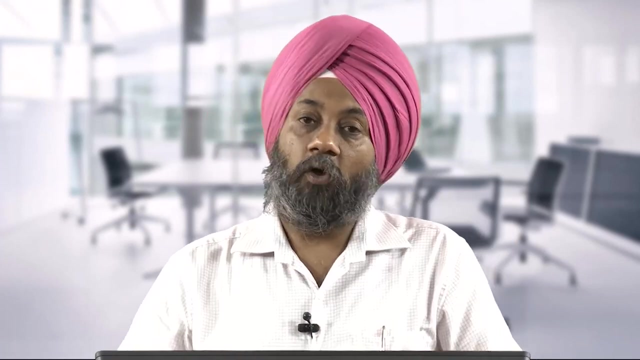 So we have to choose from a set of materials which are already available- x and y. But if we want to do modifications in our product design, if we have a new materials or a list of new materials, We have more choice in terms of changing the shape or changing the functionality of our. 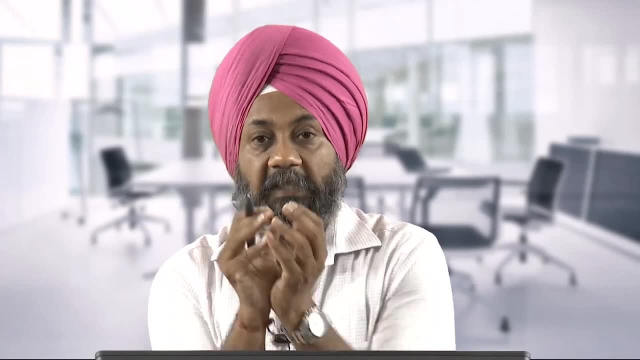 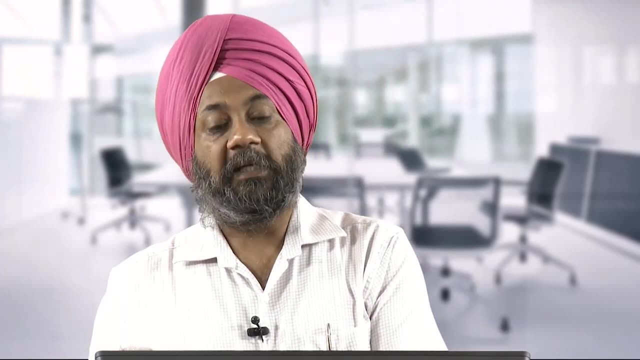 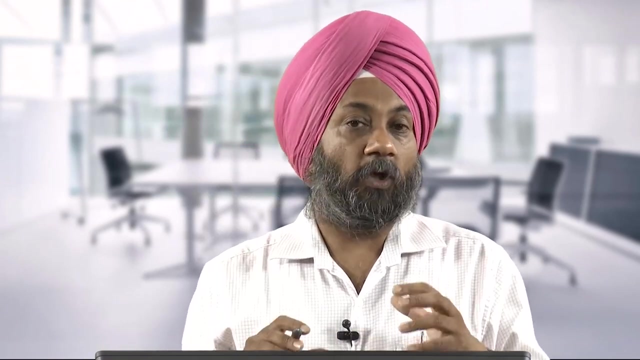 product. But if there is a limited set of materials available, we will be limited in our design thinking approach. So that is an important point that has to be kept in mind. So that is what is governing factor here, that we have to choose the optimal material. but 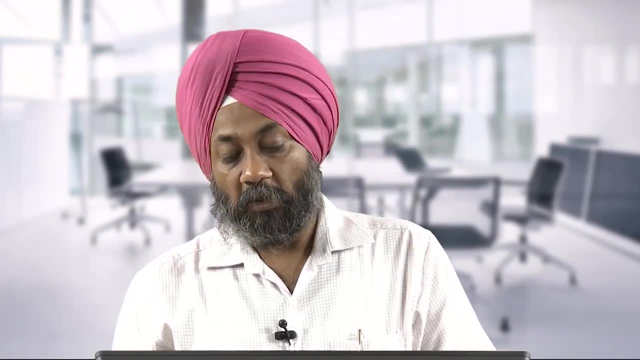 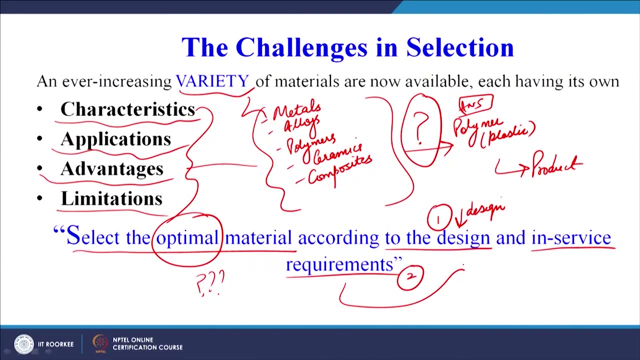 that will depend on design- On design as well as it will depend on the in-service requirements. Now, in-service requirements can be that the it is going to be used for underwater application- one important in-service requirement- or it has to be always used in sunlight only, or 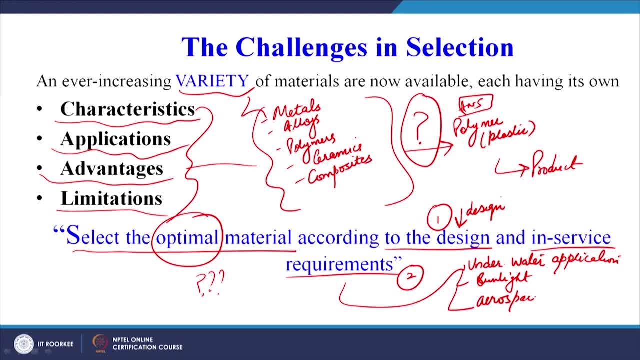 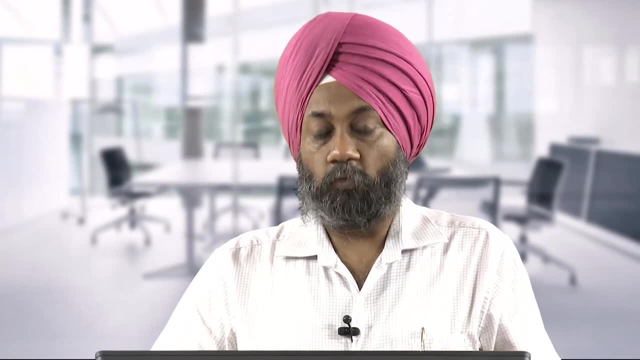 it has to be used for aerospace application. So the in-service requirement, So the in-service requirement. So the in-service requirements in aerospace applications will be different as compared to a ground surface application. So, depending upon the in-service requirement, we have to choose our material. 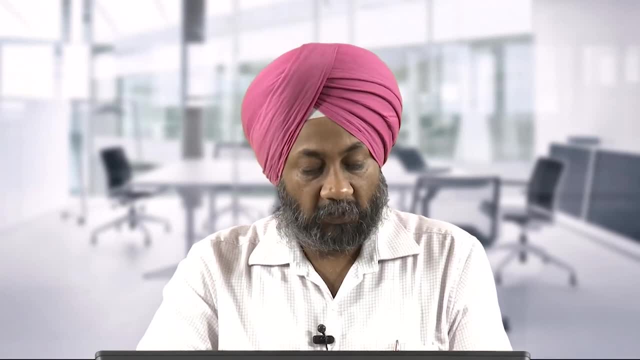 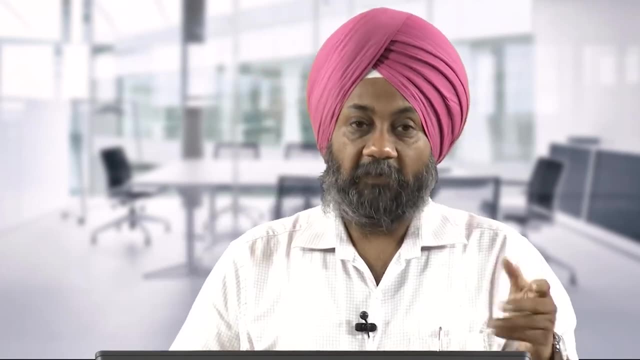 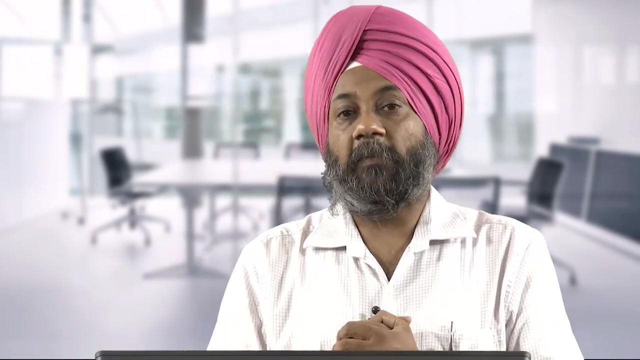 So the design and in-service requirements are the guiding factors for selecting a material for any application Now this selection will depend upon. now we have seen that there is a challenge of selection. there is a large variety of materials available. we have to choose from among those materials. 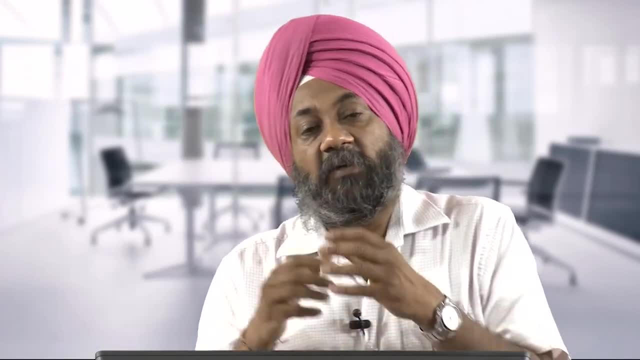 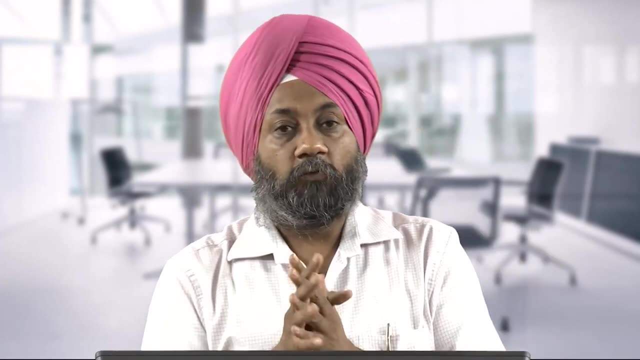 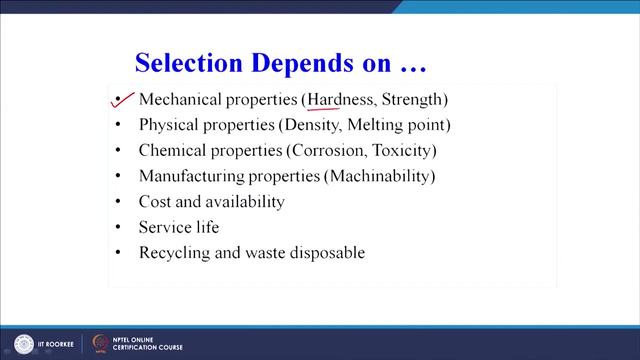 Now how to choose. we will choose based on the design as well as the in-service requirement. Now how, or what, are the quantifiable parameters that we will use for selecting the material? We can look at the mechanical properties. they are usually quantified. we have hardness. 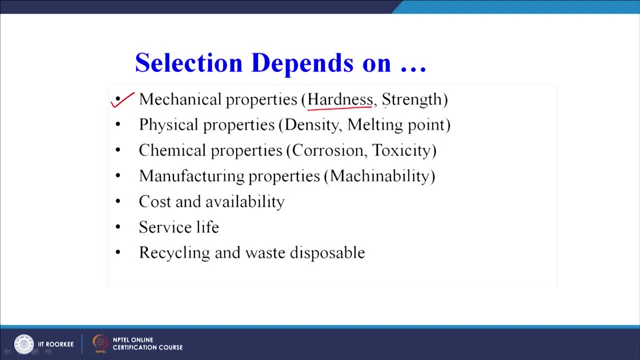 there are scales in which hardness is measured, we have strength. we can measure the tensile strength. So using the universal testing machine UTM and find out the strength of a material, Now that data sheets are already available, and if you refer back to our discussion in 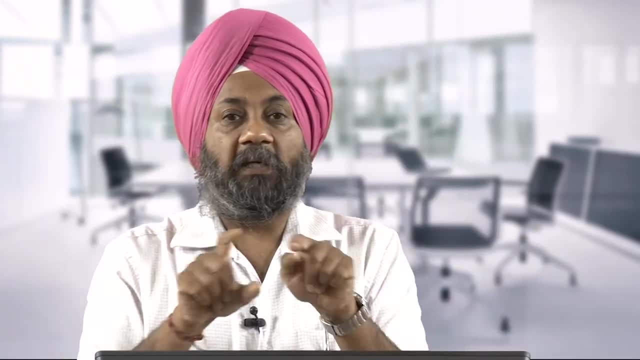 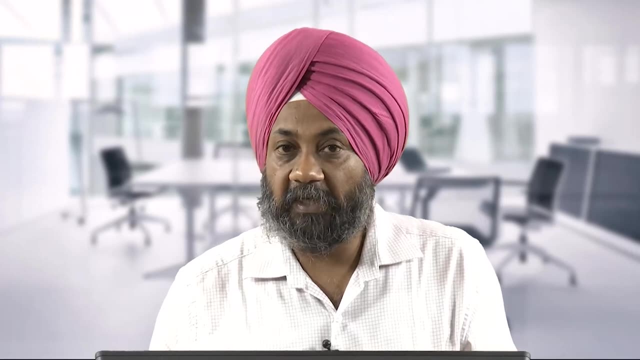 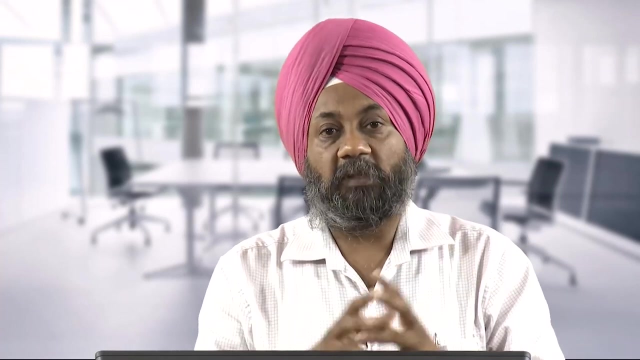 the properties of engineering material. towards the end, one data table was given in which all the mechanical and physical properties of the different metals and alloys were depicted. So those type of tables are available in which we have the quantified properties means, the values of the various properties. 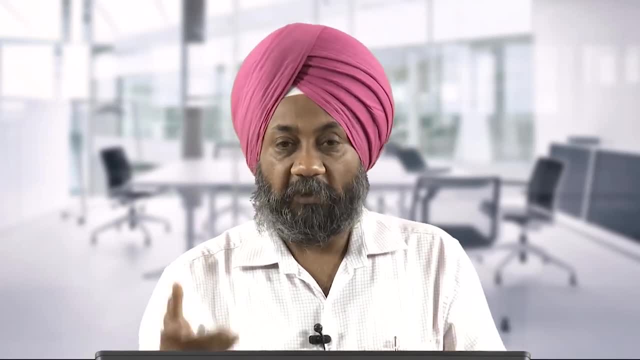 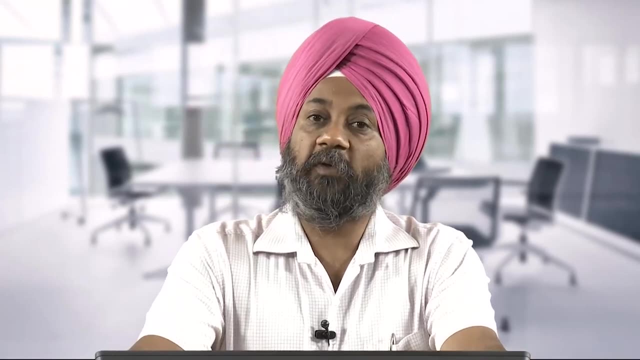 Like for steel, Steel or a particular type of steel, what is going to be the strength, specifically the tensile strength or the compressive strength or the shear strength? all those values are already available. So when I am designing the product, I will do the analysis of the product and find out. 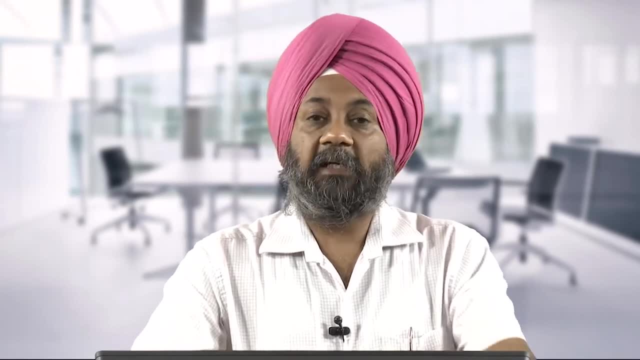 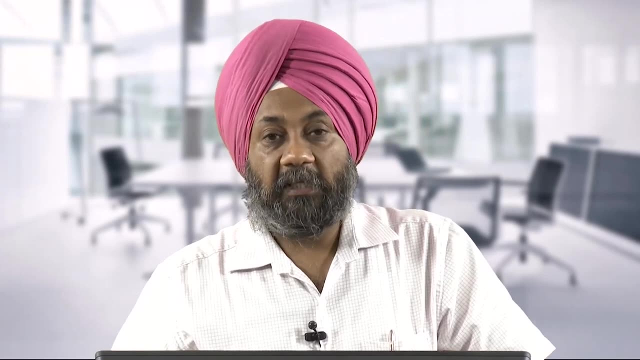 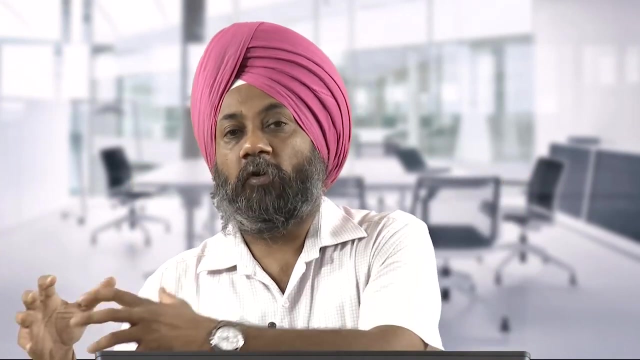 that how much must be the strength of the material that I must propose for this type of a product design, And for that I can refer back to the data book and find out that which are the materials which have the strength More than or better than the strength that is required for my product. 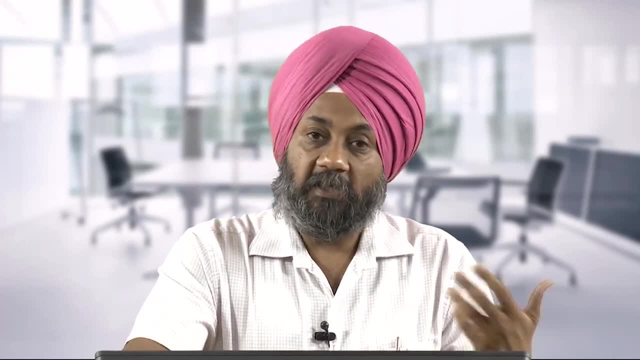 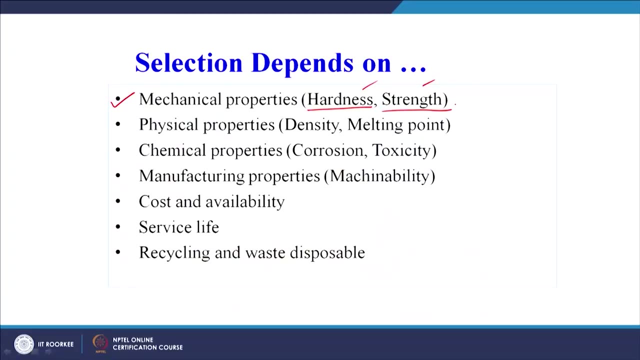 So I will definitely select the material which is having better strength. So, similarly, hardness also, and these are not the only 2 properties. we may also, depending upon the application, we may also like to look at the toughness properties of the material. In many cases, we may be interested in the modulus of the material that we are going. 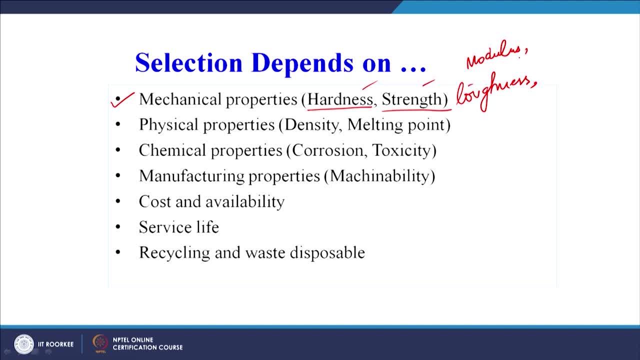 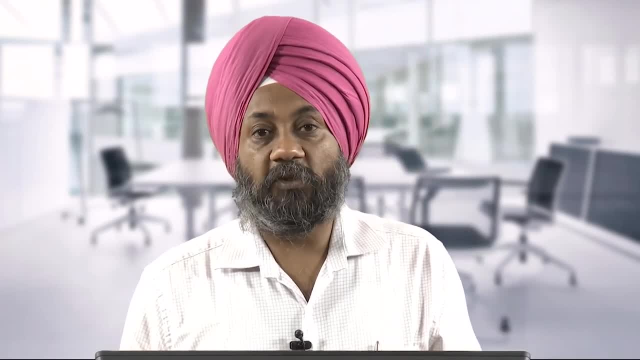 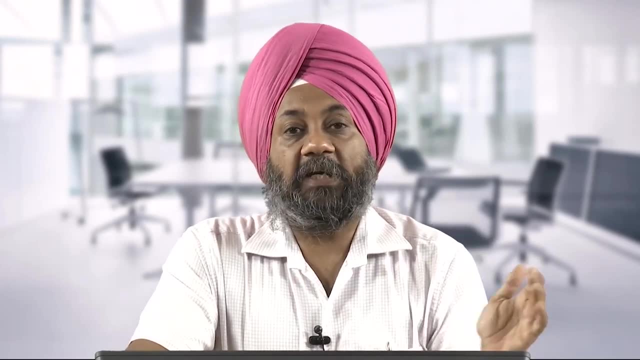 to propose For our product design. so the mechanical properties play an important role and these are quantifiable values and these are maybe mathematical values which will help us to select a material for a particular application. Some materials will automatically get screened out based on the mechanical properties because 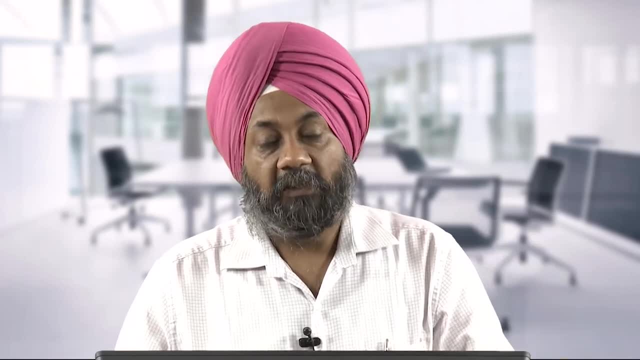 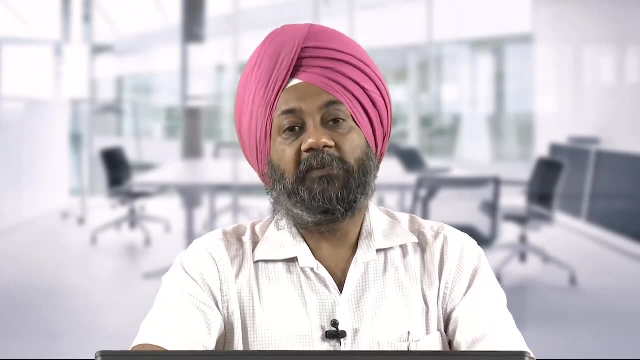 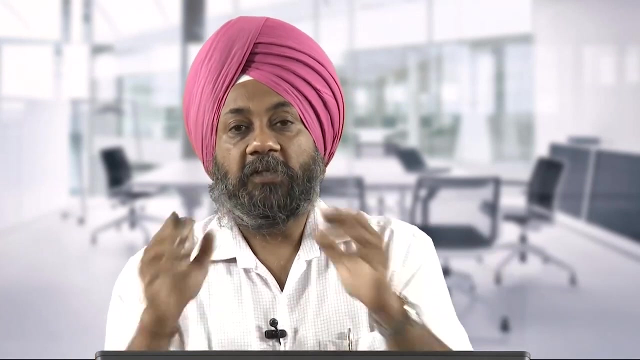 the kind of strength, the kind of hardness, the kind of toughness that we require sometime, the kind of creep properties that we require, may not be satisfied With a specific set of materials, so those materials will automatically get screened out. We will be left with a certain set of materials which satisfy the properties as per our product. 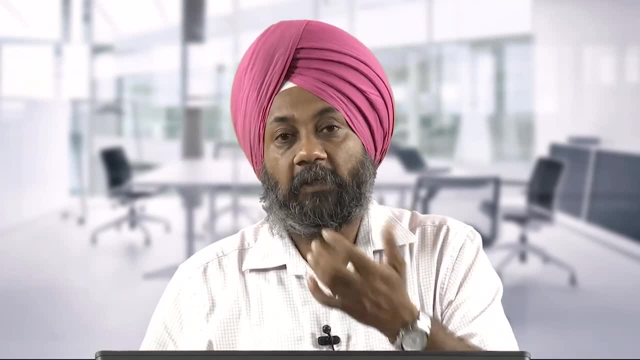 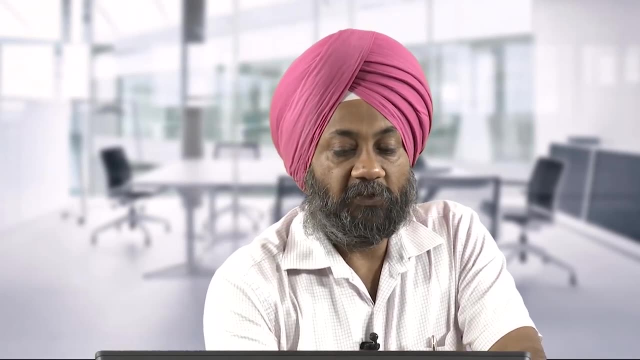 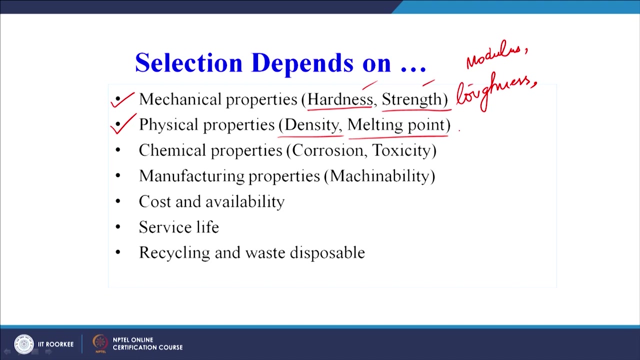 design. So that is can be one guiding parameter for shortlisting or screening the materials for our product design. The second can be the physical properties. so physical properties like density, melting point, boiling point, All these properties will help us to screen out some of the materials. we will select the 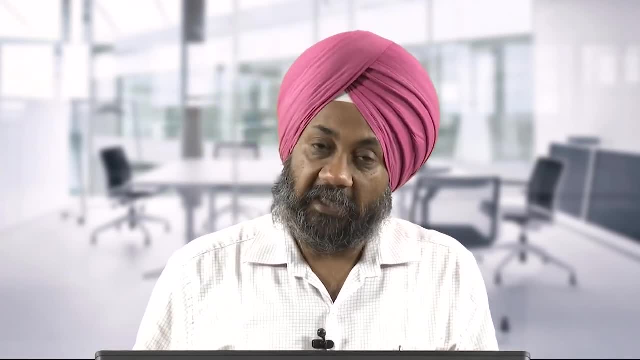 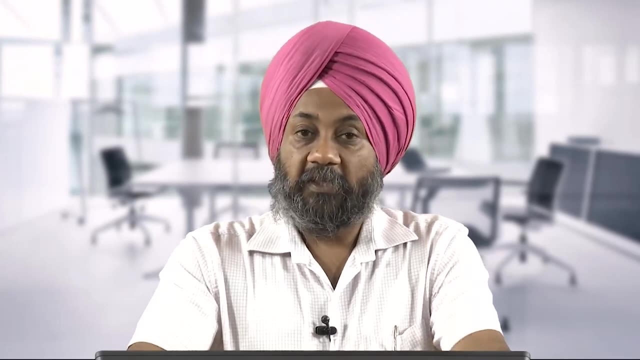 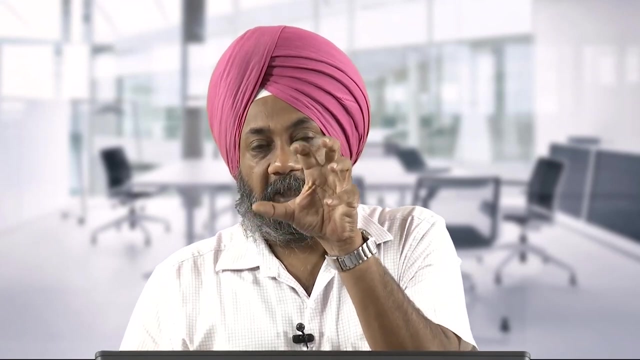 best materials which suit to our product design as well as the application for which the product is being designed. So the physical properties will also help us select the material. and if you remember just today's session, only we have seen the material attributes. they influence the shape. 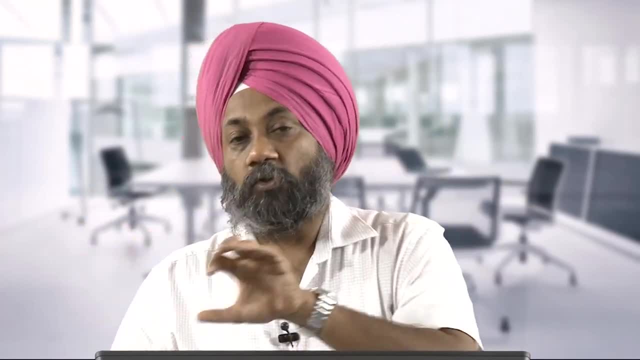 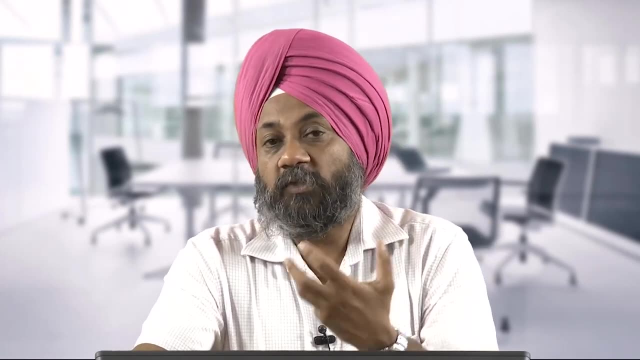 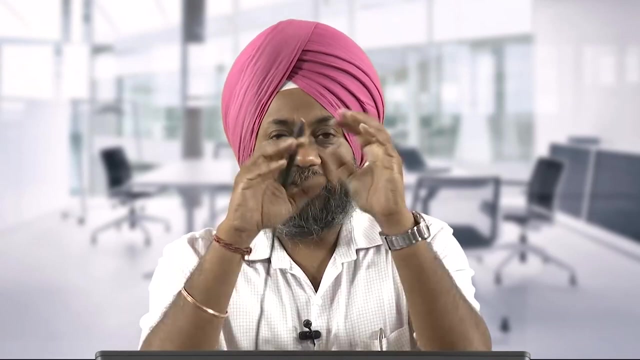 they influence the functionality, they influence the process. So Physical properties may also help us to select or define that which process we can choose for making our product design. So basically, once we select a material, it is a may be a cyclic process. we may first 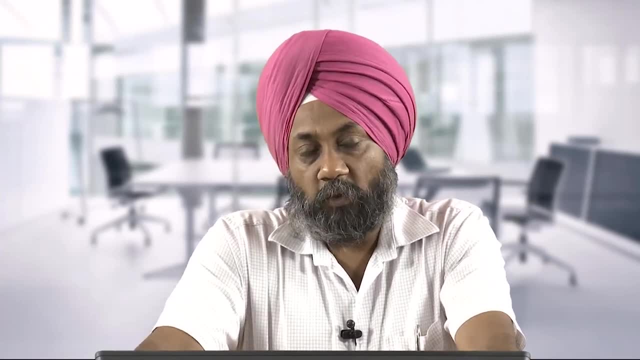 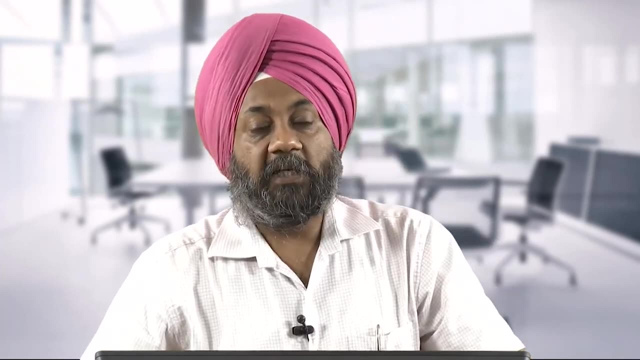 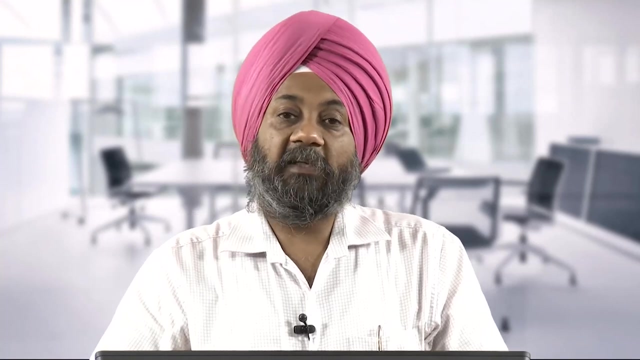 like to decide on the material and then look for the manufacturing process. or sometimes we may have to change our design because of the manufacturing facilities that we have. So We may have a product design in plastic, but we may not be having the machine which will. 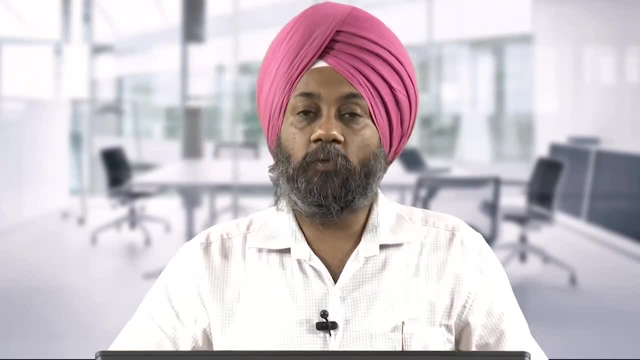 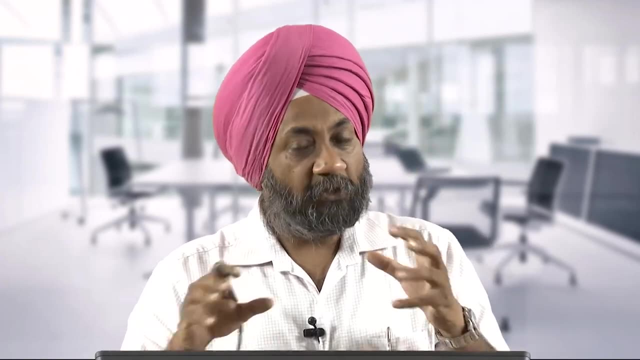 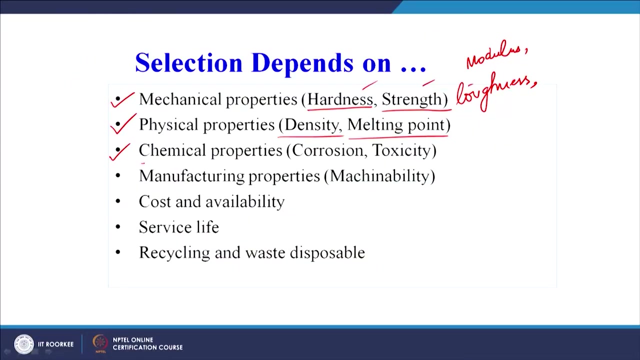 be able to process the plastic. So therefore we may also be limited, sometimes with the manufacturing facilities that the company has. So therefore, physical properties will also help us to select the materials accordingly. Similarly, the chemical properties, such as corrosion toxicity. another one can be oxidation. 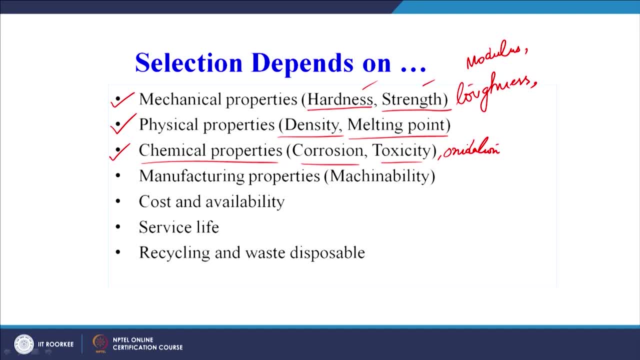 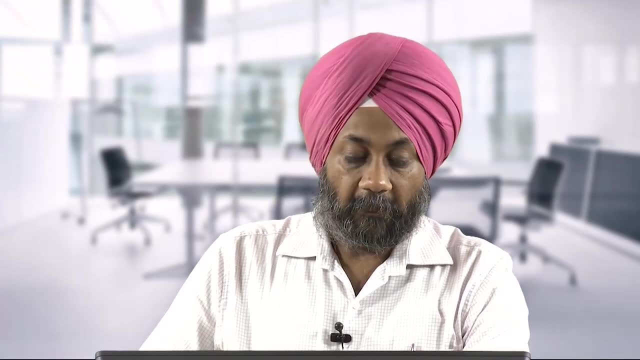 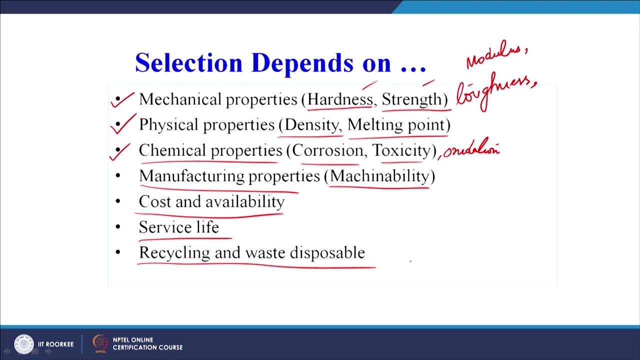 So all these properties will definitely help us to select the material. then the manufacturing properties, such as machinability. we will see there can be other manufacturing properties also, like castability, weldability, formability. So that will help us to select the materials. Cost and availability, service life, recycling and waste disposal- all these are also important. 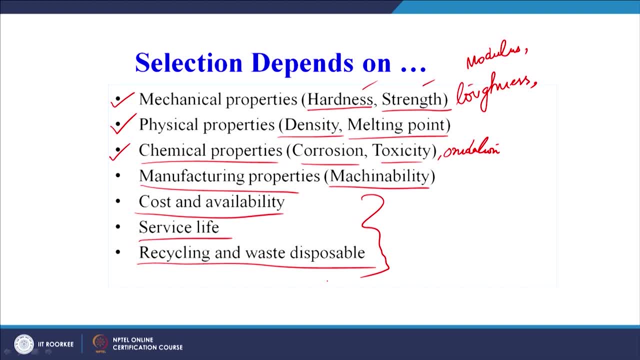 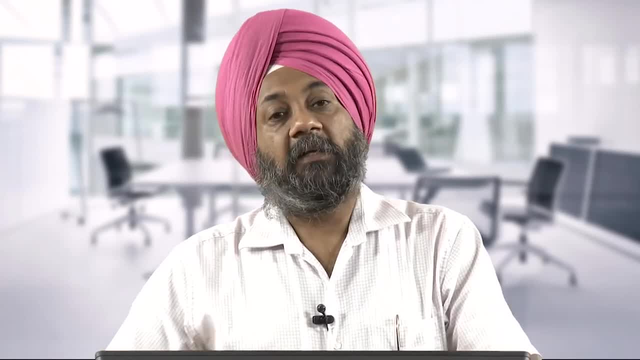 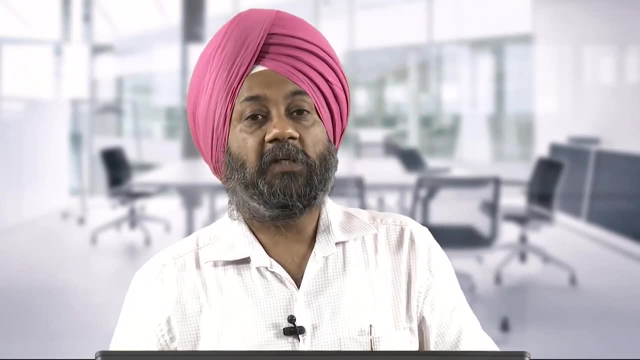 parameters which have gained significant relevance events in today's scenario. Now, waste disposal, as all of you know, is a very, very important parameter these days, and there is a talk about sustainability, green environment, green products, green processes. So, therefore, we must select materials which are healthy, which are, we can say, environment. 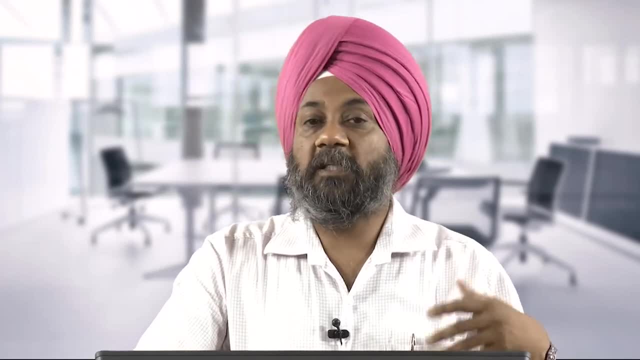 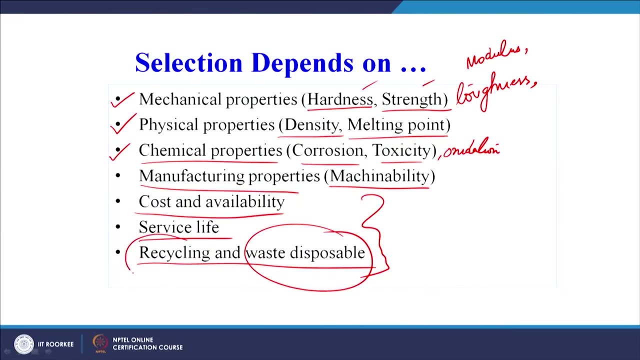 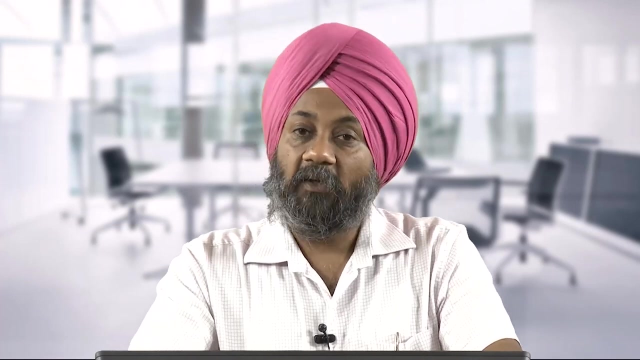 friendly, which are easy to dispose of, which we can dispose of into the environment without causing any harm to the environment. So this waste disposal, recycling are these days playing the most important role in choice of materials that we are going to make for our product design. 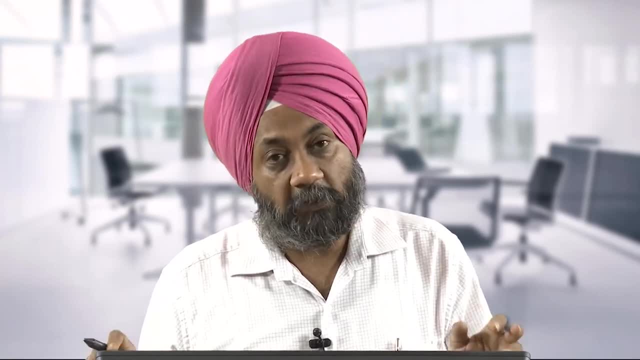 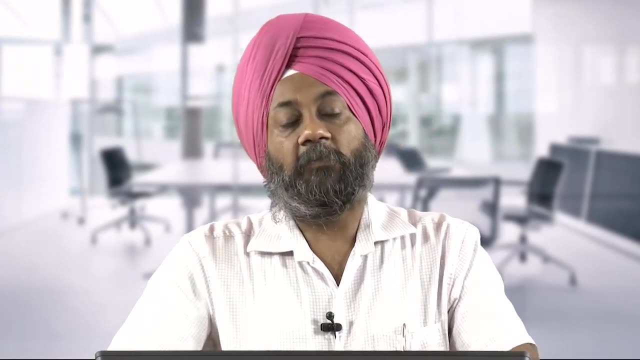 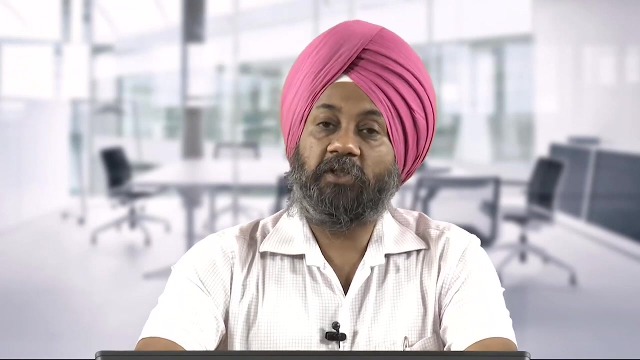 So if our product can be made or must be made with materials which are recyclable, materials which are easy to dispose or materials for which the waste disposal is not going to affect the environment. Similarly, the cost and availability is an important criteria, even sometimes the material. 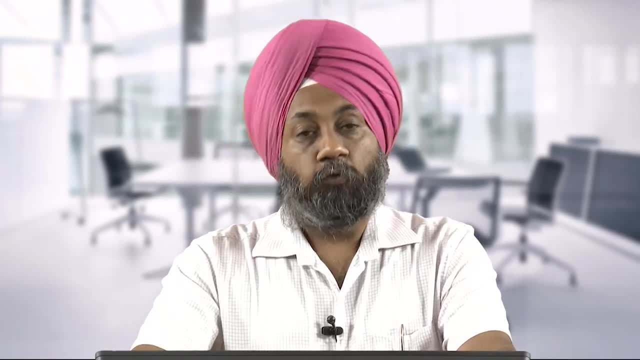 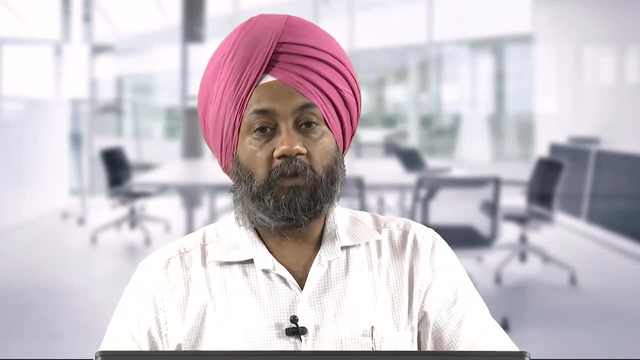 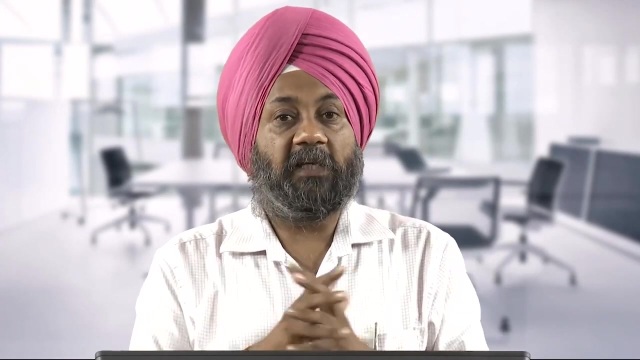 is not available, So we may be forced to select a material which is having high cost or is expensive. So these are all the governing parameters, governing, we can say, criteria which will help the designer to select a material for the product design. So let us see now summary of these. 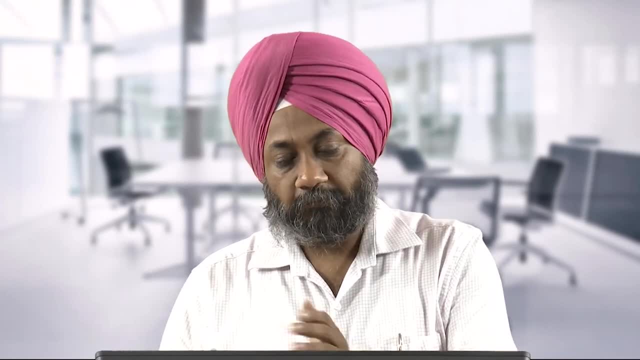 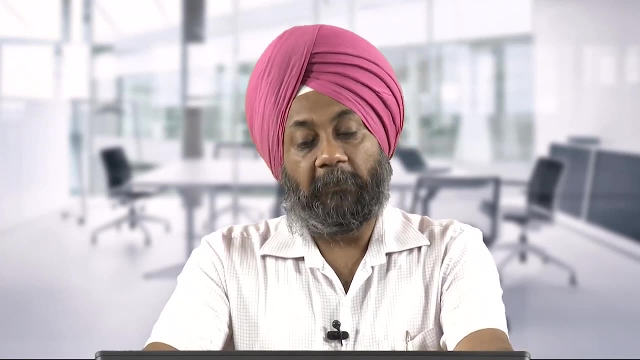 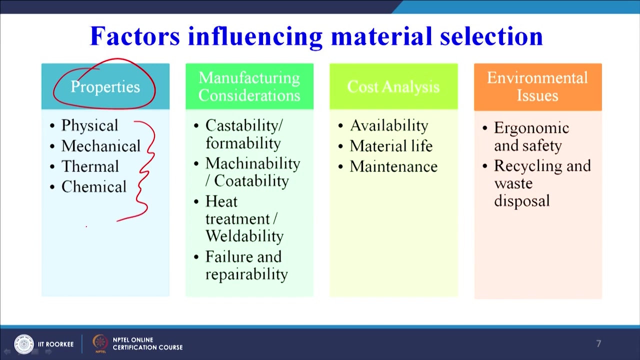 Summary of these So quickly. we will have a round of criteria or may be a listing down of important parameters related to material selection. So we can see here properties play a important role: physical, mechanical, thermal and chemical, as is clear on the screen. 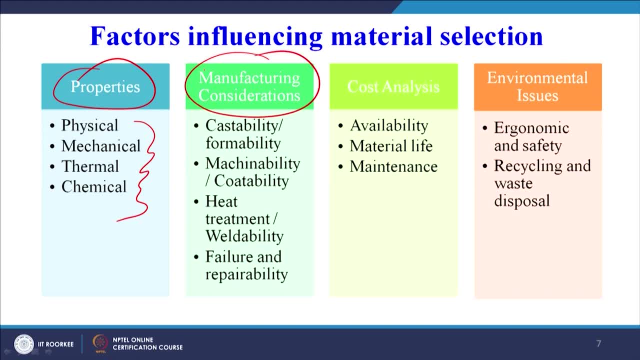 Then the manufacturing consideration. in the last slide only we have written machinability. we can also talk of castability, formability, machinability, coatability, Whether heat treatment is possible, weldability, failure and repairability. Similarly also, it was mentioned cost analysis, availability of the materials. what is the? 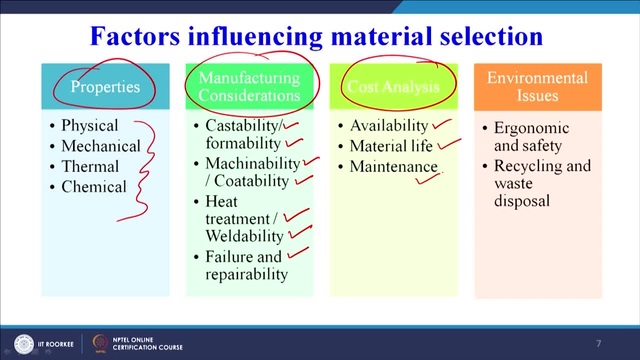 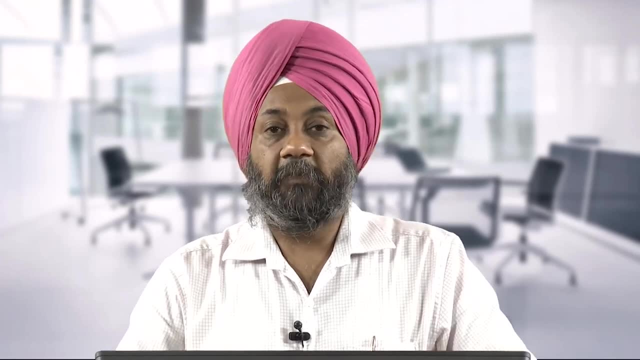 life of the material. what type of maintenance is required for the material? especially for underwater applications, frequent painting of the surface of material may be required, So we can choose a engineering material which does not require frequent painting or maintenance. requirement for the material may be less. 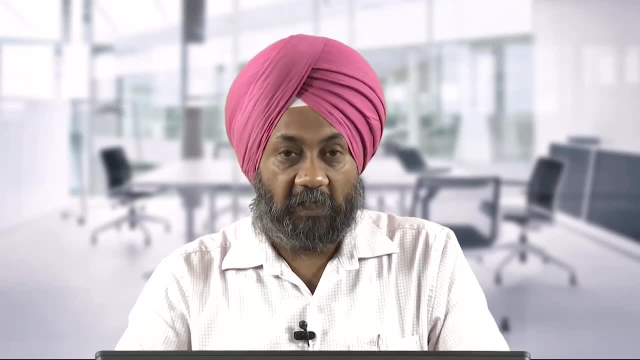 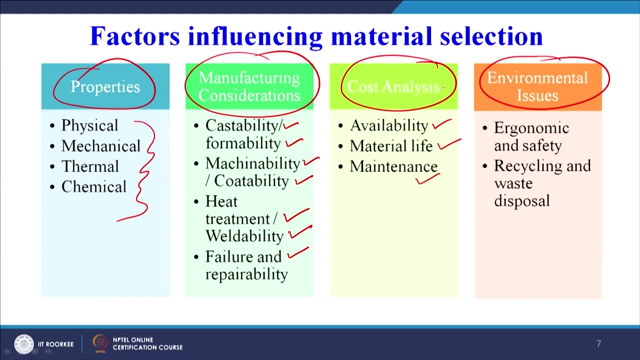 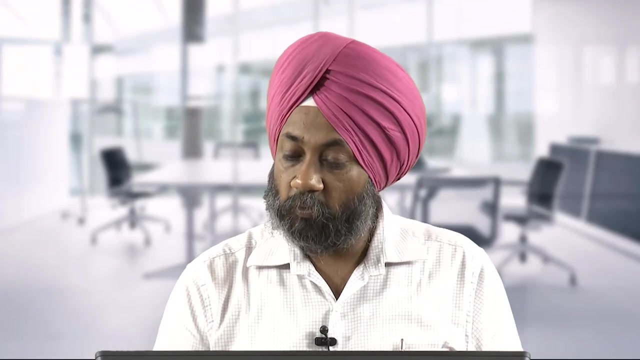 So for specific applications like underwater, we may choose material which do not require much maintenance. And the last part was environmental issues. I already addressed related to the waste disposal. I already addressed related to the recycling. So we have to see that the materials, like ergonomic and safety, must be ensured. 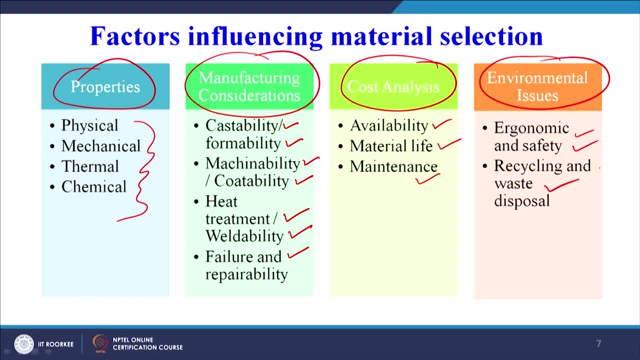 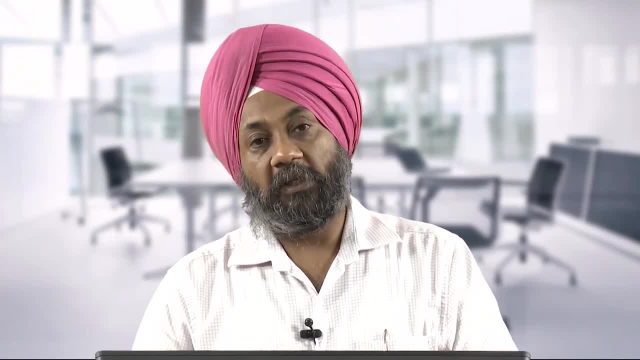 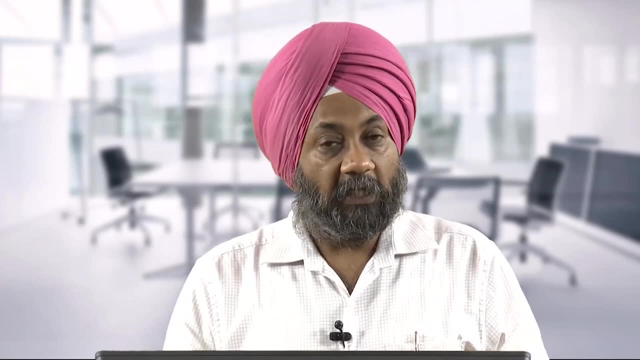 Similarly, recycling and waste disposal also play a very important role in defining the choice, In defining the material that we are going to use for making our product. So I think, with the time constraint of 30 minutes for each session, I will conclude the today's session here and the next session quickly. we will have quick review of all these. 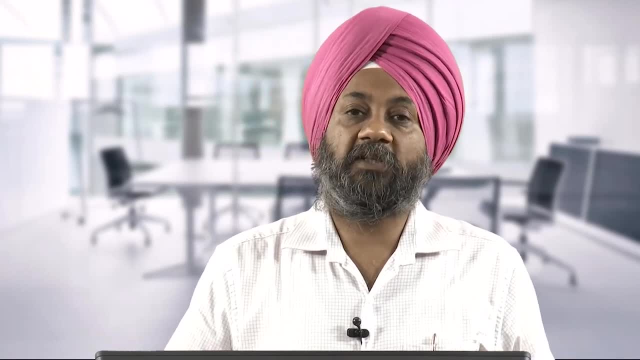 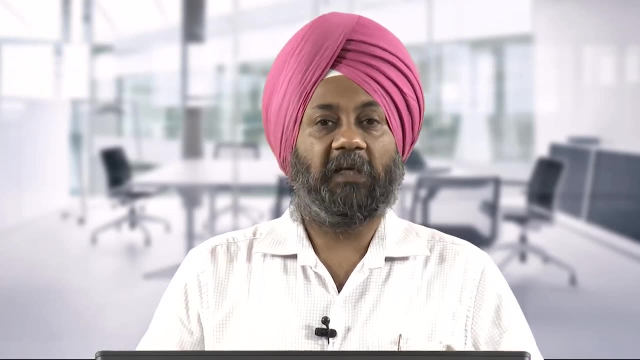 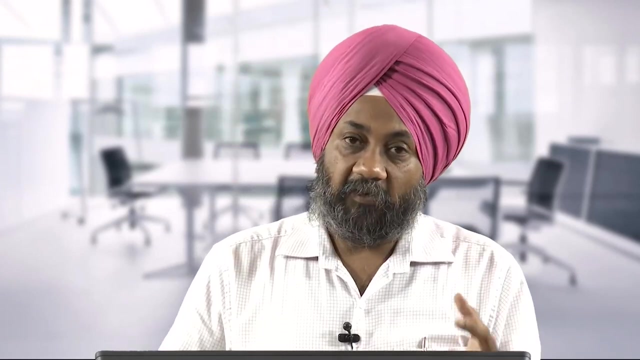 properties, and then we will try to carry forward our discussion related to a step by step or a systematic process for selecting a engineering material with the help of a case study. we will try to understand. So today's conclusion is that we have tried to find out the importance of selection of